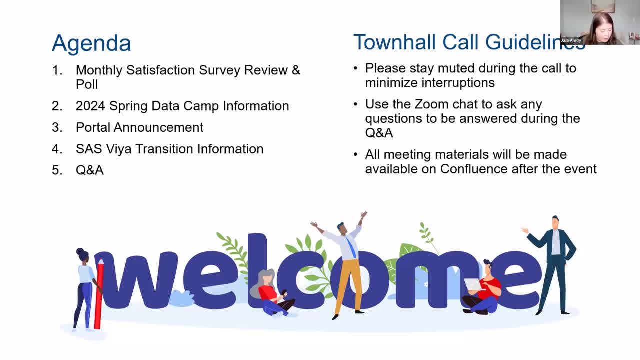 the meeting materials available in Confluence after we wrap up. So now let's cover our agenda. We are going to kick things off today with our monthly satisfaction survey review and then our poll, And then next we're going to be covering information about the 2024 Spring Data Camp and then an announcement on the DNA portal. 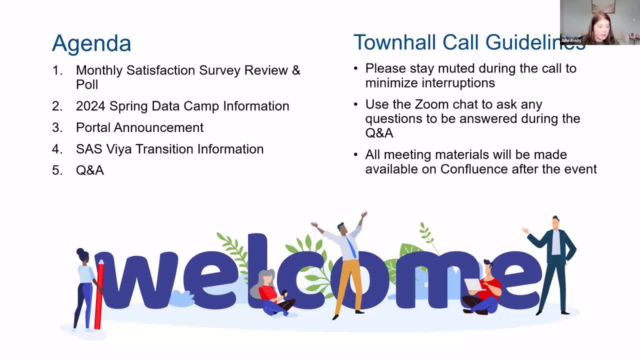 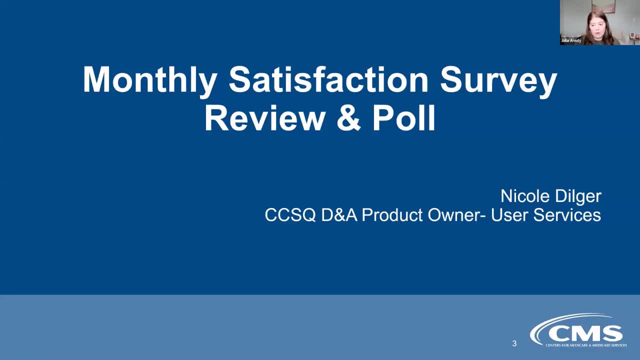 and then SAS VIA transition information And finally, we'll be wrapping up today with our Q&A portion of our call. Okay, so I'm going to pass things over to Nicole to kick things off with our monthly satisfaction survey. Hi everyone, And real quick. before I get into this, I know we had the maintenance page. 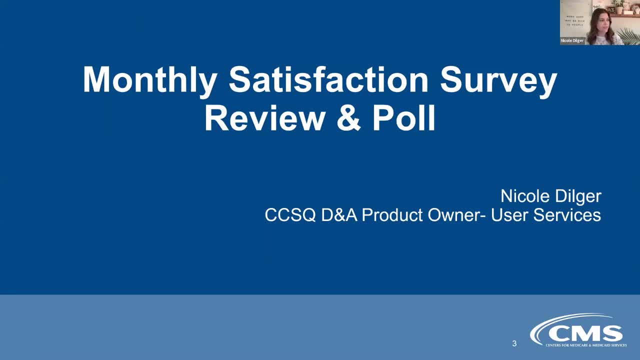 up before and I just wanted to say that we just sent a communication out, about 15 minutes ago, that there's going to be a SAS outage on Friday. tomorrow, April 12th, from 8 pm to 11 pm Eastern. 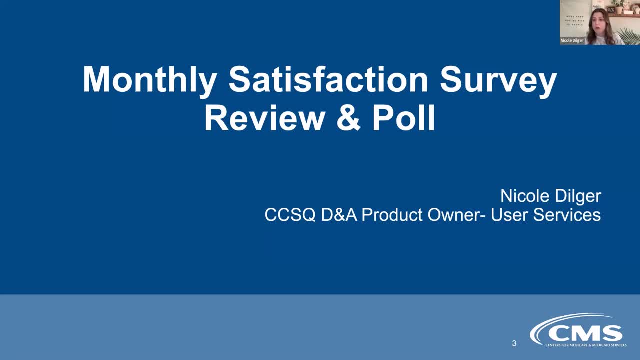 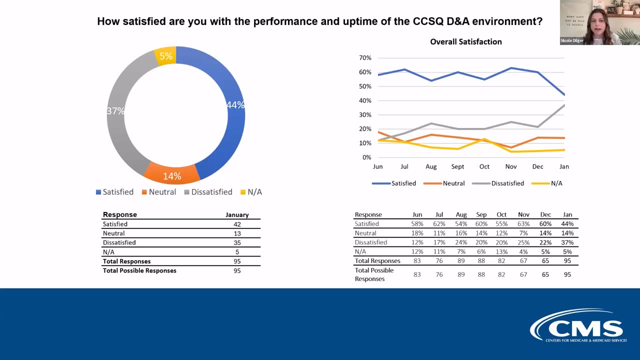 So just wanted to make sure everyone saw that or knows about it, in case you didn't see it yet. All right, now we can get into the monthly satisfaction survey review and poll. Oh, and also I don't know if I introduced myself, So if you're new here, I'm Nicole. 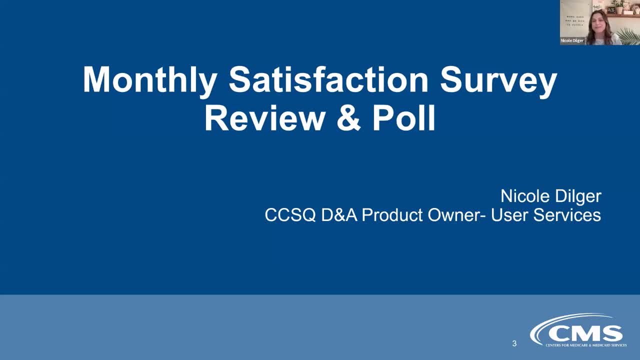 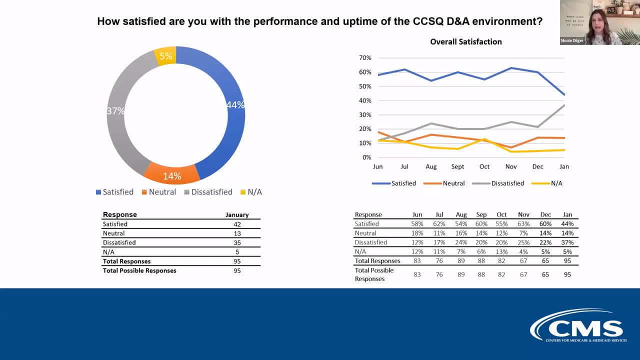 Dilger and I am the CCSQ DNA product owner for user services. All right, so we are going to be reviewing the survey results. As a reminder, we did not have a town hall in March, So these survey results are actually from the town hall that we last had in February, where we asked the survey participants to rank. 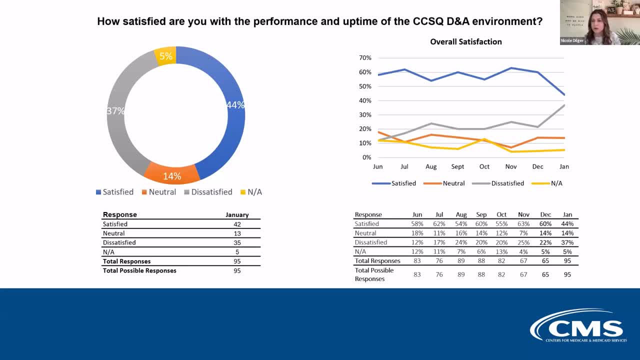 their satisfaction for the month of January. So just in case anyone is wondering why it is showing January, that is why, When we take today's survey, we can do that for the month of March, and then this will be Updated then for the next time we meet. So I just wanted to go through that. 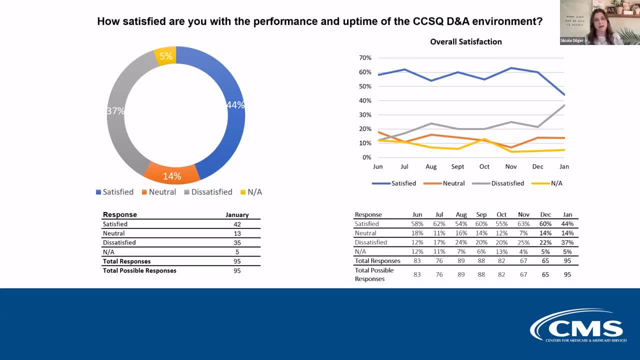 All right. so how satisfied are you with the performance and uptime of the CCSQ DNA environment? For the month of January, we did have a decrease in satisfaction, with an increase in the dissatisfied category. You can see we had 44% satisfied, 14% neutral, 37% dissatisfied. 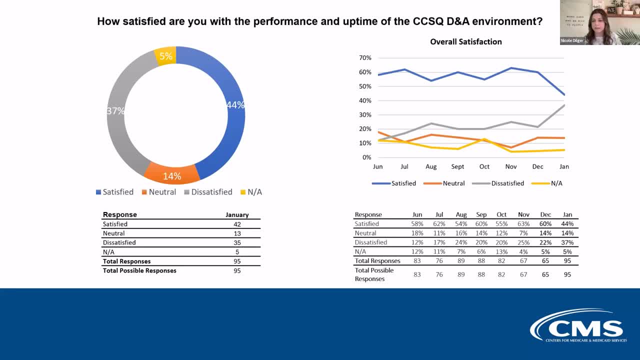 and we had More participation in the last town hall. We had 95 responses, So we saw the most participation we have over the past six months in that survey. So thank you for those that participated. We can go ahead and go to the next slide. 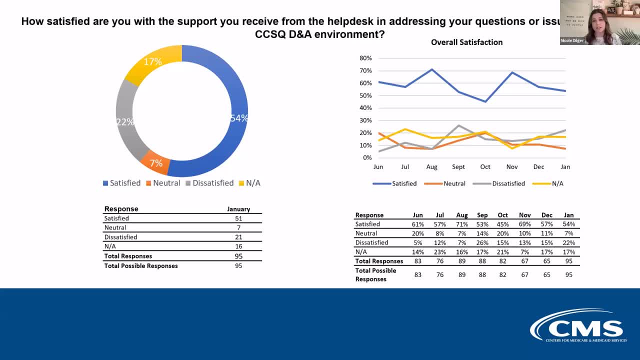 How satisfied are you with the support you receive from the help desk in addressing your questions or issues with the CCSQ DNA environment? Once again for the month of January we had a decrease in satisfaction: 54%. We had 7% neutral, 22% dissatisfied, 17%, NA for that one and once. 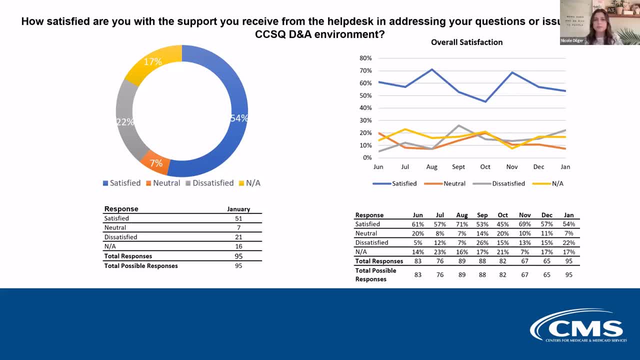 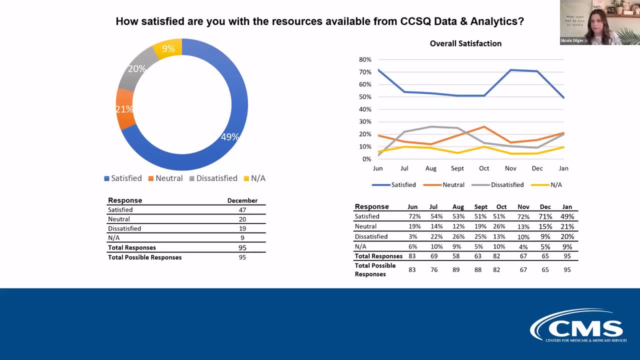 again 95 participants. You can go ahead and go to the next one. How satisfied are you with the resources available from CCSQ data and analytics? We had a decrease of satisfaction for the month of January and again an increase in dissatisfaction. You can see in the scores. 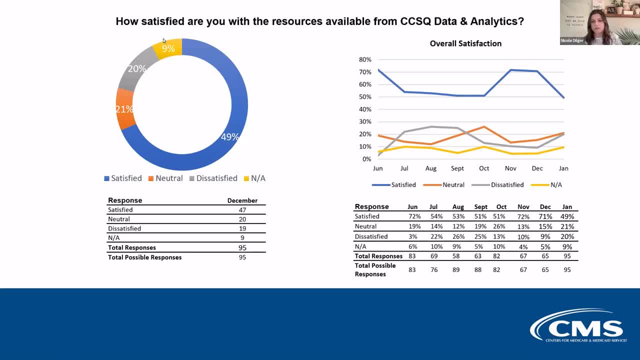 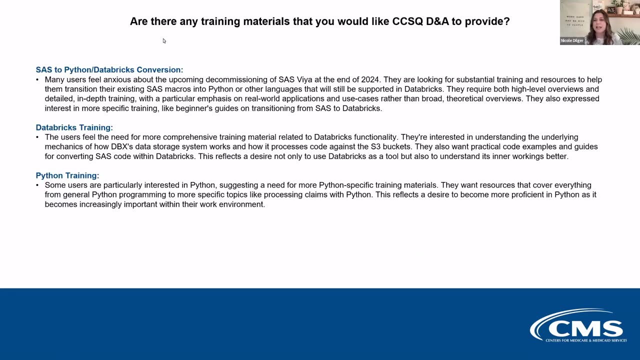 there- 49% satisfied, 21% neutral and 20% dissatisfied- And I'm going to talk a little more about what we are doing because of those results, If you want to go ahead and go to the next slide. So in our survey, we ask about training materials. What would you all like to? 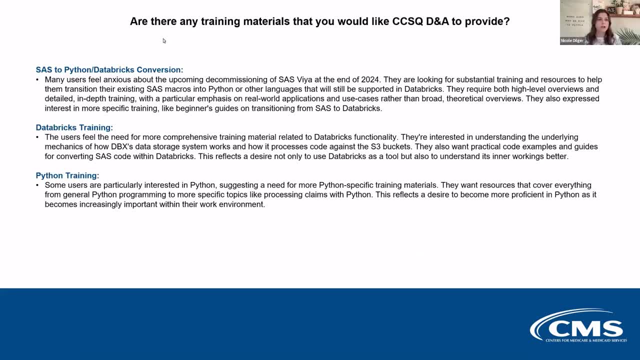 see, We got some great feedback in regards to SAS, to Python, slash, Databricks, conversion training or tools, Databricks training specifically, and then Python training, And because of that, we'll be going into this a little later when we go over the SAS transition information. 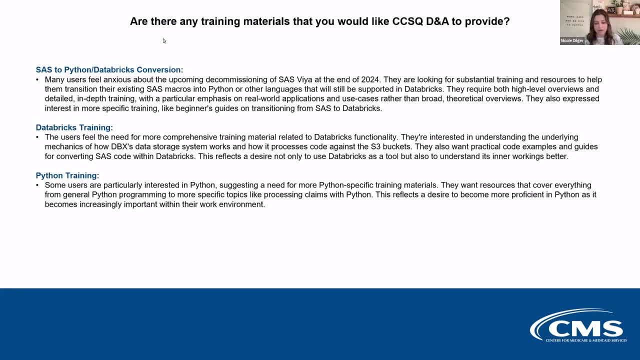 of how we're going to be taking this feedback that you've all provided and acting upon that to give you all the resources you need and are asking for. So just wanted to go over that and we'll talk more about that when we get into the SAS transition portion of this meeting. 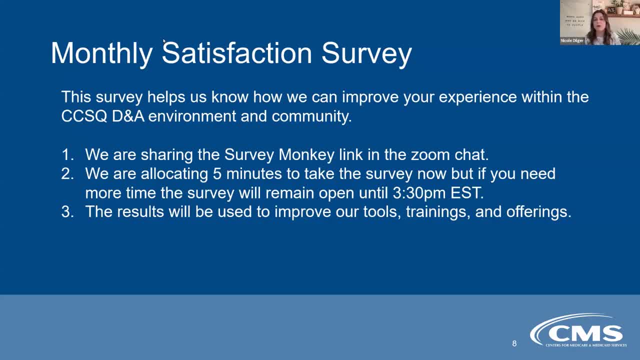 You can go ahead and go to the next slide. Okay, So with the monthly satisfaction survey, most of you are used to doing this in Zoom, but we are going to be doing it a little differently. moving forward, If you participated in the monthly satisfaction survey, you're going to be doing it. 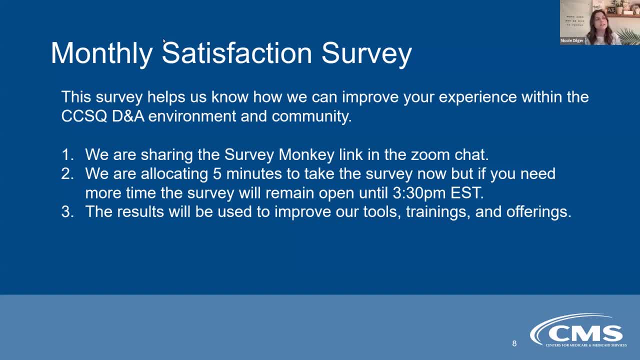 in two of our most recent surveys related to SAS transition, You would have noticed we used a tool called SurveyMonkey and we are going to continue to use that, moving forward for the monthly satisfaction survey as well. So this will be a little different in that we are going to be 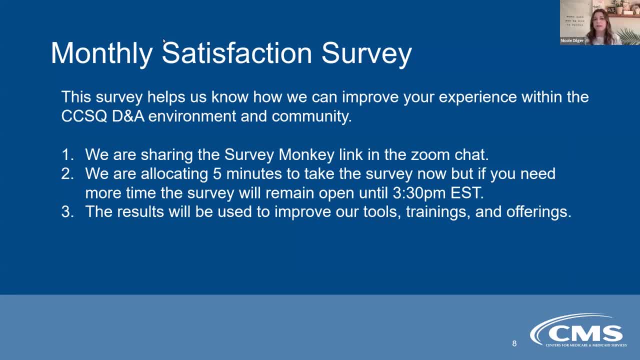 sharing the SurveyMonkey link in the Zoom chat. When you click on that, we're going to allocate five minutes for you to take the survey now, But if you need more time, we're going to leave the survey in the Zoom chat. So if you need more time, we're going to leave the survey in the Zoom chat. 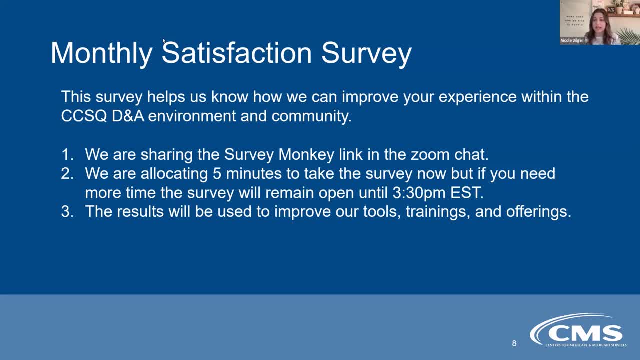 We're going to leave the survey open until 3.30 pm Eastern today so that you can have that additional time after the meeting if you'd like to take a little more time in answering some of the open-ended questions. But obviously the results will be used then to improve our tools trainings. 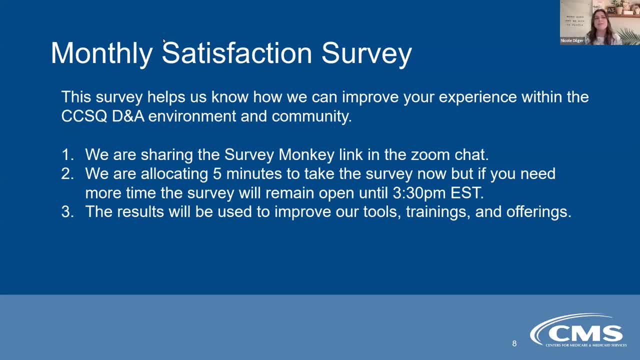 and offerings. And then I just want to give a reminder: if you are not a user of the CDR or Databricks or SAS in connecting to the CDR, you do not have to take this survey. We just want to make sure that we are able to take the survey. So if you are not a user of the CDR or Databricks, 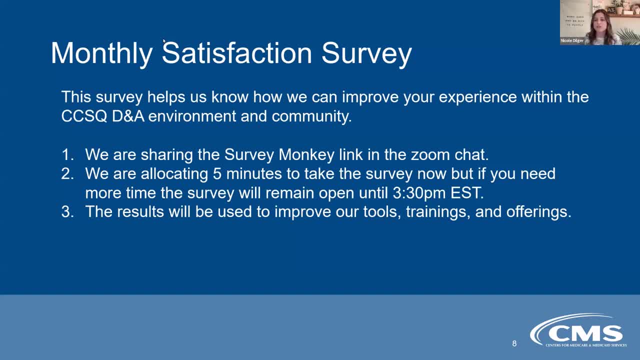 or SAS in connecting to the CDR or Databricks or SAS, we are not getting a ton of NA answers for folks that aren't utilizing those services. So if you can go ahead and find that link in the chat and take the survey, we'll pause here for five minutes and allow you to answer those questions. 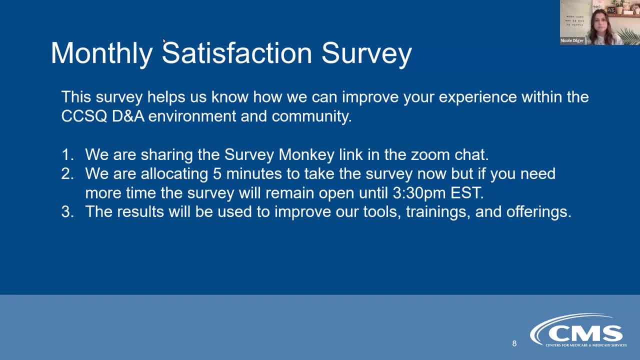 So if you have any questions, we'll pause here for five minutes and allow you to answer those questions. So if you have any questions, we'll pause here for five minutes and allow you to answer those questions. Just a heads up: we're about one minute into the survey, giving us four minutes remaining. 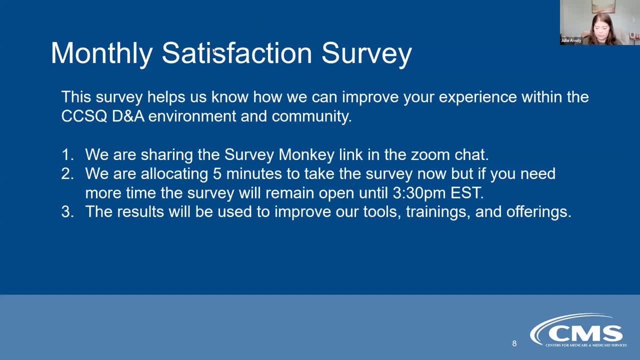 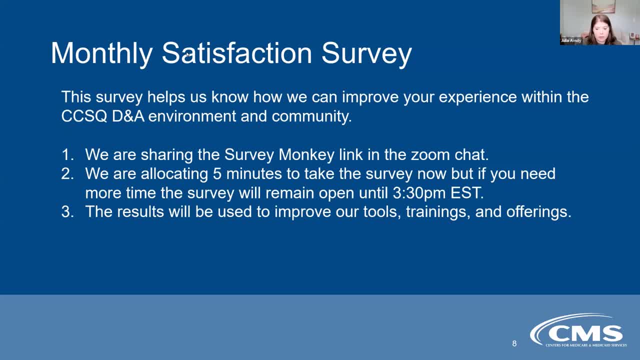 At this point we're about halfway through our survey time. And then just a reminder: as Nicole said, if you don't finish, you can certainly finish that after our call today and then submit. And then just a reminder: as Nicole said, if you don't finish, you can certainly finish that after our call today and then submit. 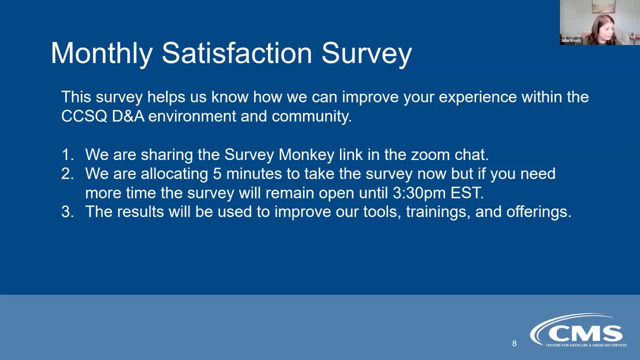 It will stay open until 3: 30 pm. Thank you, We have one minute remaining in our survey time- 30 seconds. Okay, we have about 10 seconds remaining. please finalize your thoughts and, if not, just wrap up after our call today. 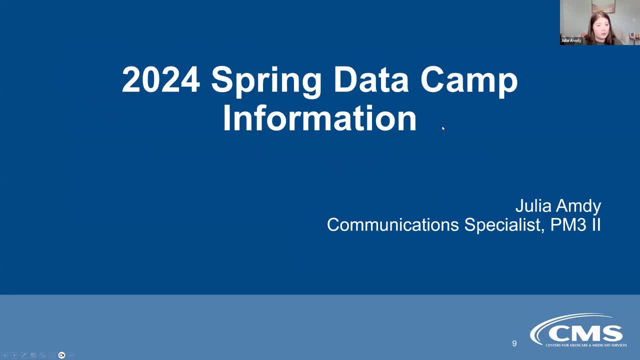 Okay, Okay, My name is Jolene Amdie. for those of you who don't know me, I'm a communications specialist on PM 32 and I'm going to be sharing some information today, as well as facilitating our town hall, on the 2024 spring data camp. 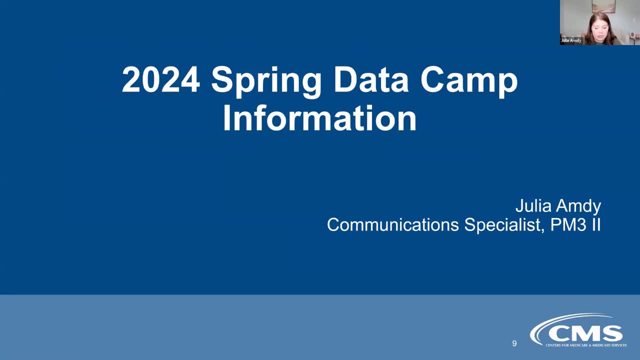 So we're going to kick things off first with a video and they'll definitely provide some additional information. but the data camp is happening this May 15 and 16 from 1pm to 5pm each day and within those days there will be sessions. the first day we'll have five. 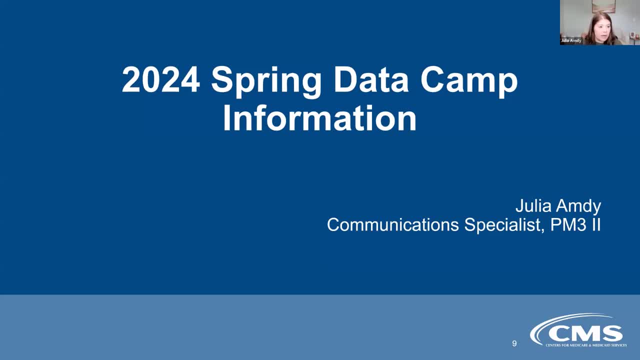 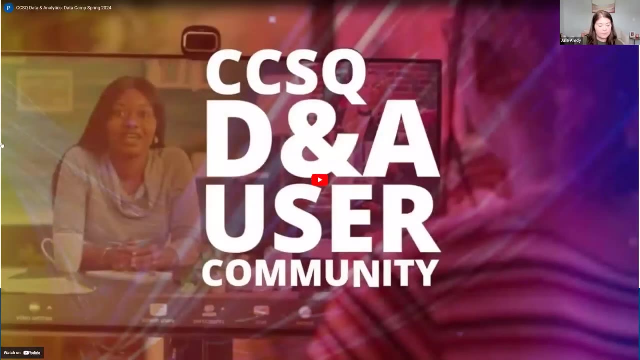 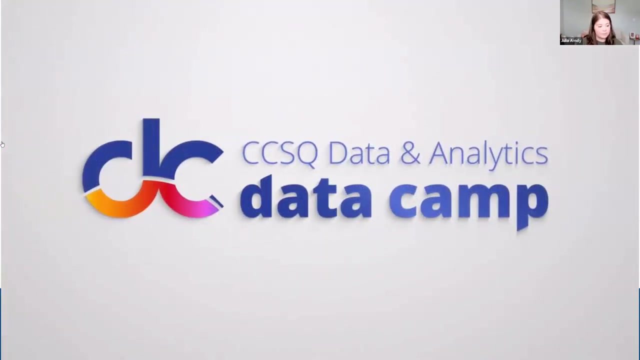 sessions. the second day we'll have four sessions And then, after a video, today I'm going to be showing you the confluence space where those sessions currently are housed and to give us some additional information and context. On May 15 and 16,, the CCSQ data and analytics team will be holding our sixth CCSQ data camp. 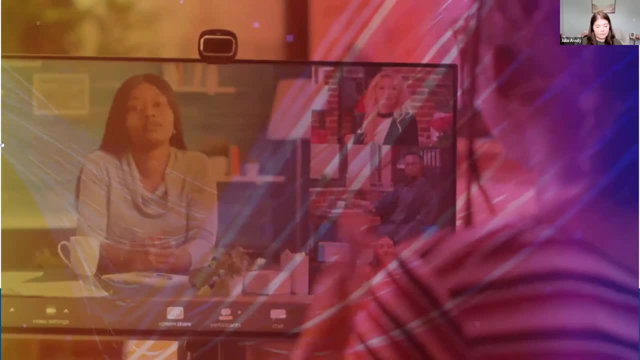 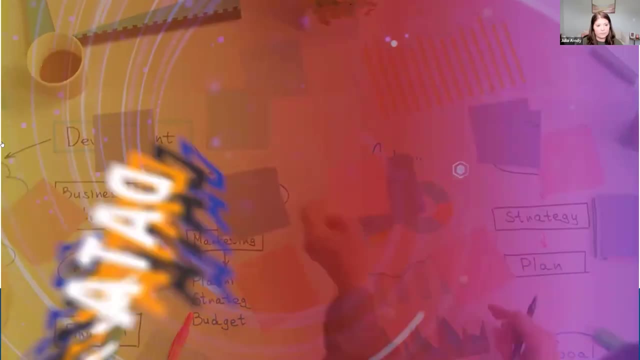 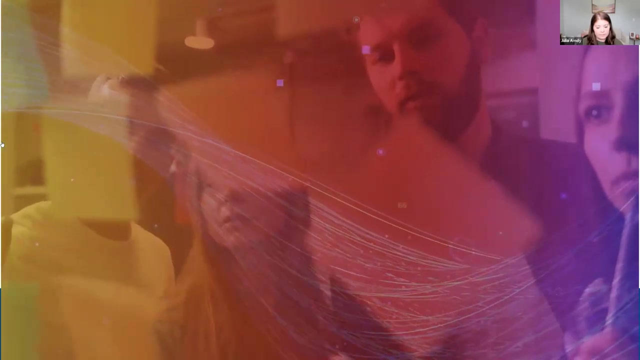 Okay, A multi-session event focused on educating the CCSQ DNA user community. The mission of the CCSQ DNA team is to encourage the community to come to the data, as it is vital to build and utilize centralized, robust and reliable data and analytics solutions. 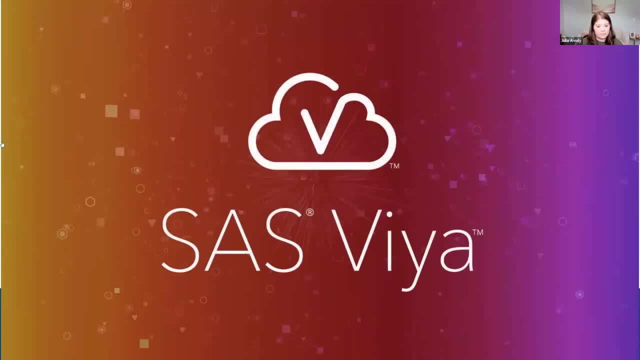 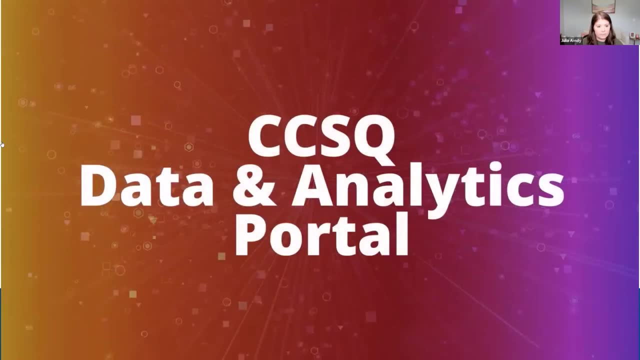 During this data camp we will be exploring sessions on the SAS Viya, transition Databricks, QuickSight and the CCSQ data and analytics. We will conclude the spring 2024 data camp with a session centered around CCSQ's future. 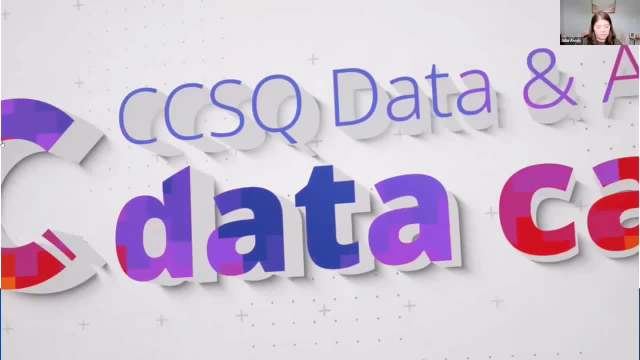 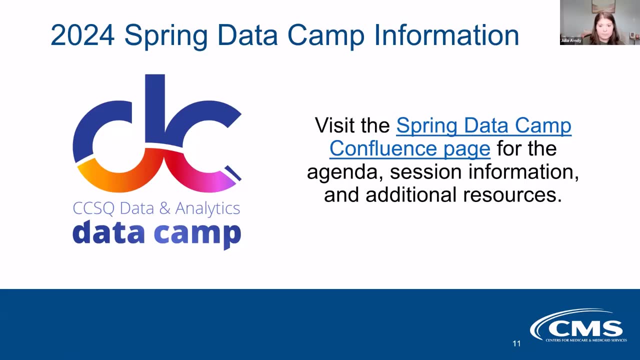 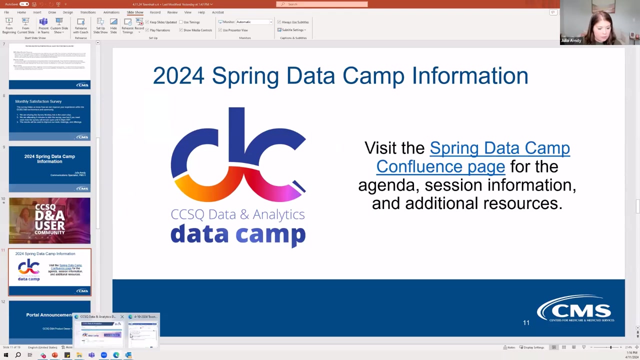 vision for the roadmap. Visit our site today for session and invitation information. We hope you can join us. Okay, so now pivoting and getting over to that confluence space. Okay, so this is the data camp. We're going to be looking at the data. 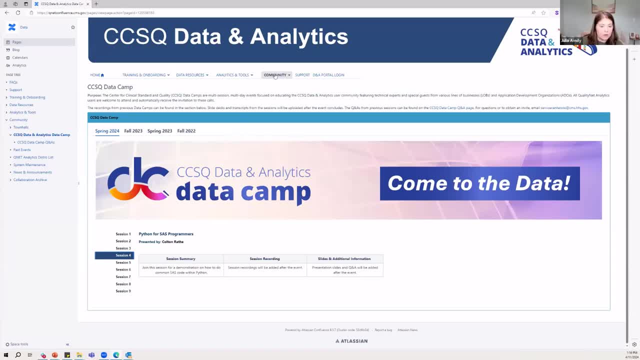 Okay, This is where our data camp information is housed. You can find it under our community tab in our DNA space and confluence. In addition, there's our town hall information, if you need that as well. So, scrolling over, there's our tabs for our past data camps as well, because I know sometimes 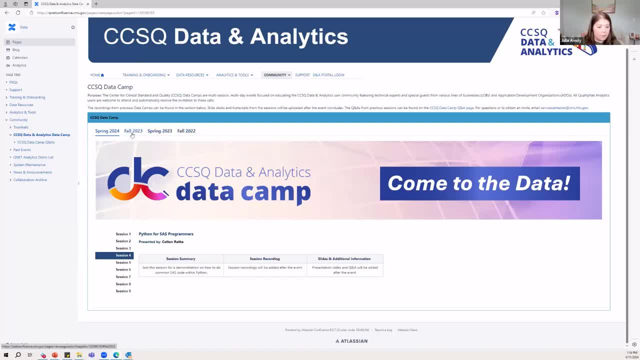 we get information or questions regarding information on that with previous sessions. So you can actually see we still have the session recordings from prior data camps. So the spring one we're getting right now we're kind of carving out information still with our session summaries. 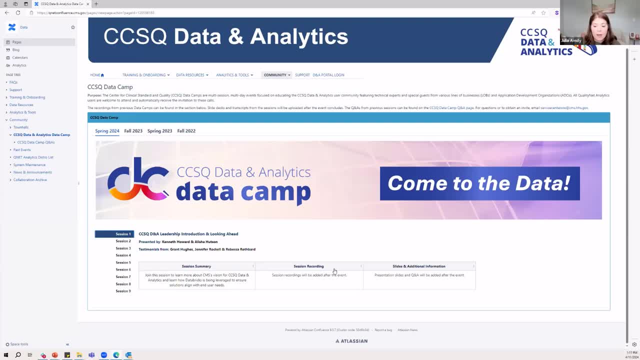 Our recordings are obviously going to be available after the sessions wrap, And then we'll also be updating the slide decks in this space as well, And then the Q&A from each session. just like town hall. it'll work the same way. We're updating that as well. 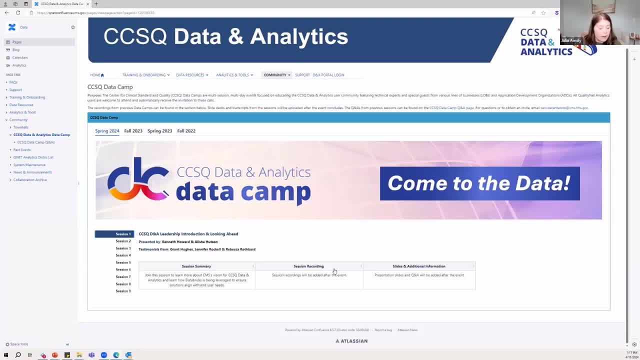 Prior to the sessions, though. this year- something new based on feedback we got last year at our survey, which is exciting- We're going to have notebooks available for those sessions that are including demos. Those will be available prior to data camp. 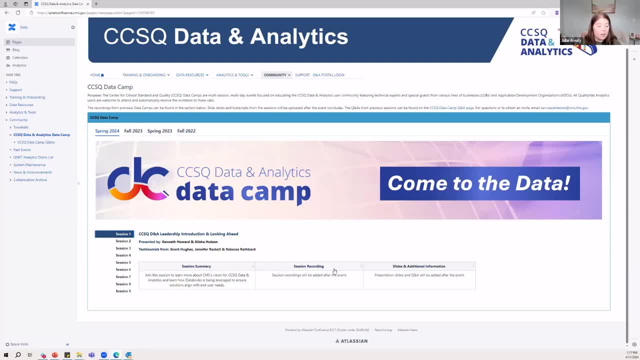 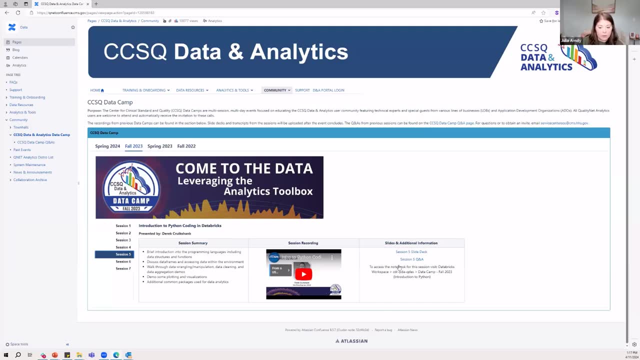 So we'll be sending information out with how to access them, But in addition, they're going to live here in this space, here, where you can see. like for the fall, for some of the ones that had the notebook available, it gave information on how to access that. 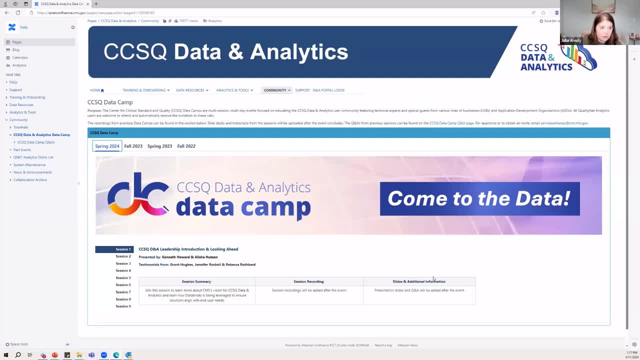 So it'll look pretty similar for spring, but that's going to be available prior to data camp instead of afterwards. We'll be sending out email communications and Slack communications as well, when those things are available to download and get started. So looking at. 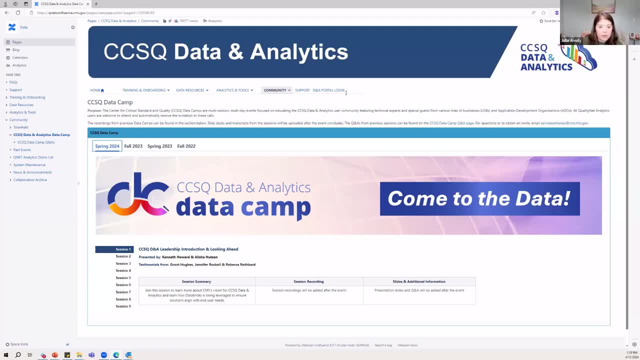 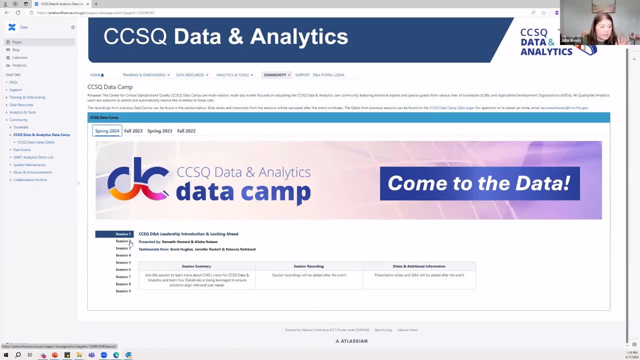 Oh, and then we did send out the invite earlier this week. If you have any questions, or or to obtain an invite if you did not receive one, you can email the help desk here and then. So now, just looking at our sessions, day one encompasses the first five sessions, so that 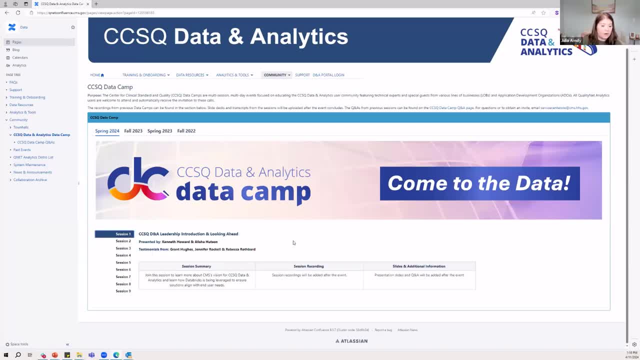 would be this first one which is going to be kicked off with Ken Howard and Alicia Hudson, And then also we're going to have some testimonials from the DVA team. So that's going to be looking at like a leadership introduction and looking ahead. 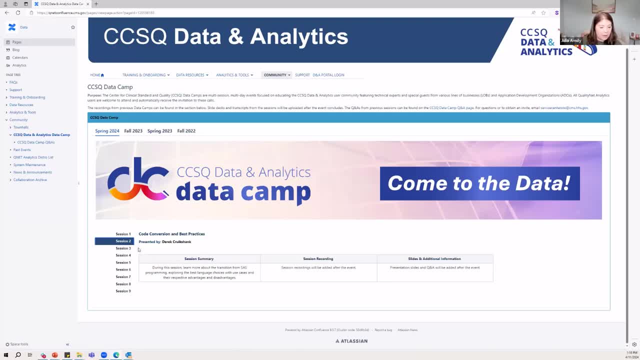 Then next we're going to have code conversion and best practices with Derek, a public portal demo, which I know we've been getting a lot of questions and excitement regarding the DNA portal, And Nicole is actually going to be giving us some more information there today. 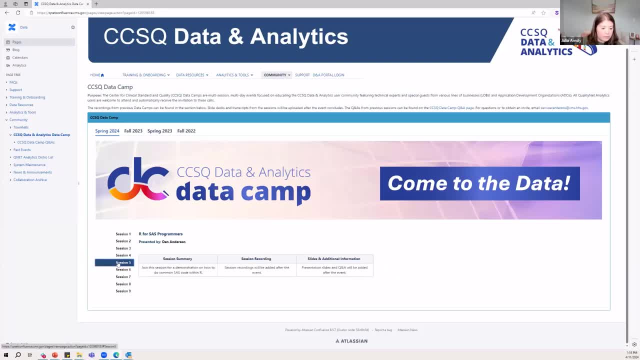 And then the next one is Python for SAS programmers from Colton, And then our last session for day one will be R for SAS programmers from Dan. And then, moving into day two, we'll kick this off, And then our last session for day one will be R for SAS programmers from Dan. 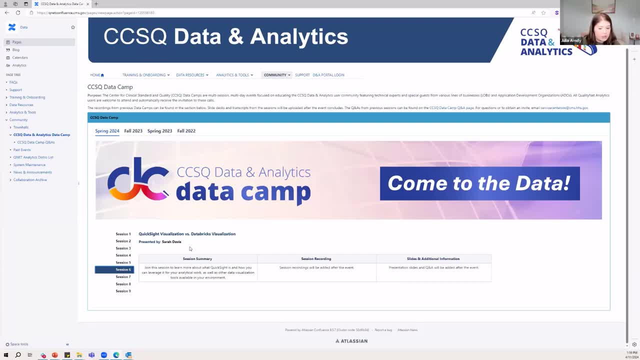 So that's going to kick things off with QuickSight visualization versus Databricks visualization, Comparative qualitative analytics capabilities, NLP, and then that one- we're going to be getting some more information soon as well, So that's exciting. And then data claims are presenters- TBD for that. 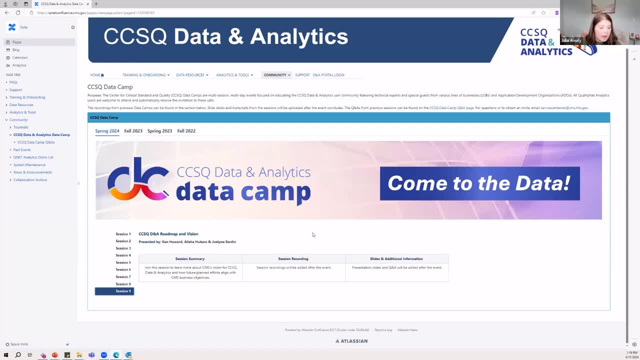 And then the CCSQ DNA roadmap and vision. So that's kind of a wrap which is a little bit different from last year as well. So our intro session is going to be kind of kicking things off and where are we going, And then I'll look back at this past year. 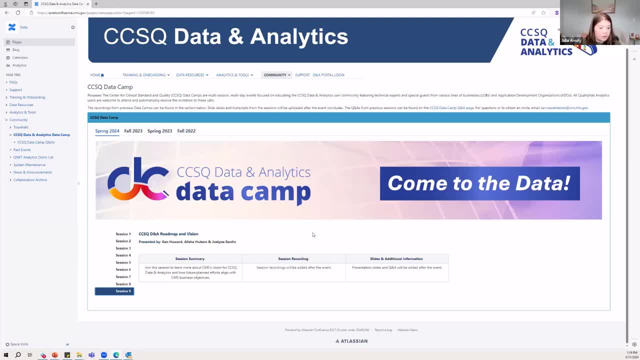 And then the last session is going to be kind of the vision for the future And that will be presented from Ken Howard, Alicia Hudson and Justina Sarveen, And I think those are sessions. right now. We're continuing to add information as we get it and as presenters are giving us materials and resources. 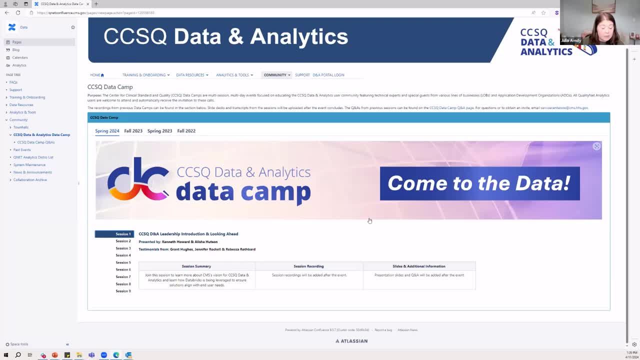 So those will definitely be coming available to our Confluence page page page. So please keep an eye out and keep checking back, And then we'll be sending out Updates via email and Slack, So look out for those as well, as we have new information and resources. 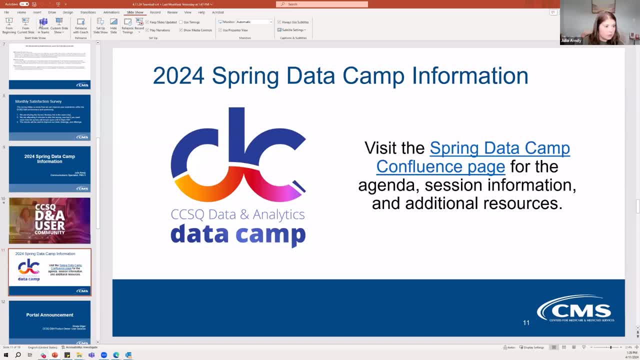 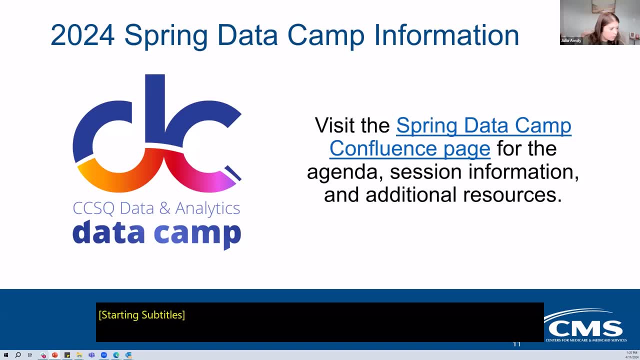 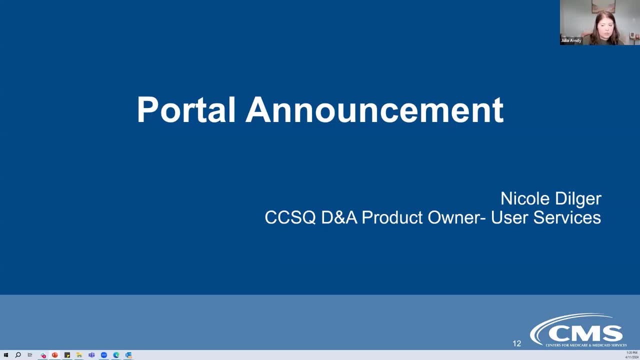 Okay, So toggling back to our presentation. Okay, So now I'm going to turn things back over to Nicole for some portal updates. Yes, And I am filling in because our portal is is out of the office right now. So I am going to just give a little bit of information about the exciting announcement for public portal. 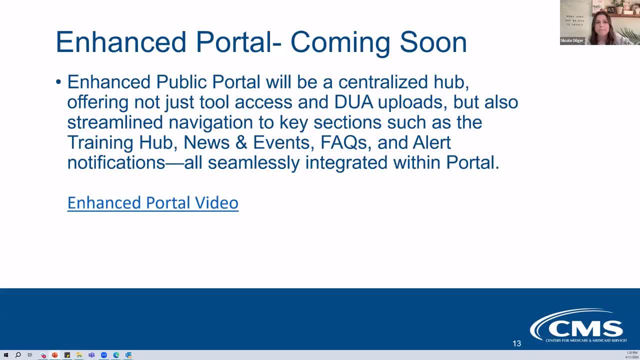 If you can go ahead and go to the next slide, Julia. So you probably saw the communications going out that we are excited that we're going to be launching the enhanced public portal. This is scheduled for For tomorrow afternoon evening, ish time frame. 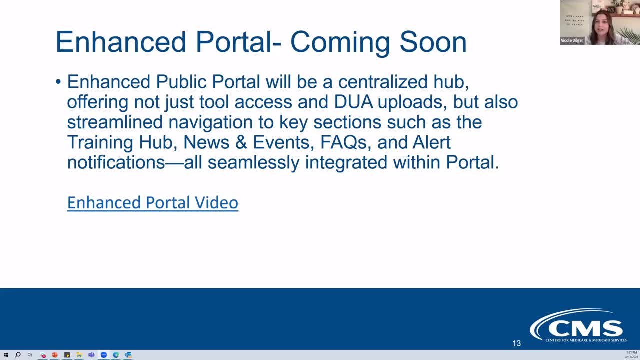 So Monday morning when you come in, this will be available for all to take a look at. the enhanced public portal is going to be a centralized hub Offering not just tool access and DUA uploads, which are currently available now in portal, but also streamline navigation to key sections such as the training hub. 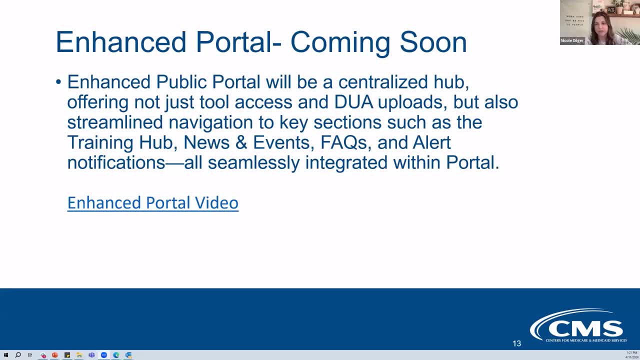 News and events, FAQs and alert notifications. So currently we have a lot of this information on confluence, but now it is going to be available in the enhanced portal And we're very excited about this, as it is very user-friendly. There's a great search function where you can go in and search for training or knowledge-based articles or any news and events that you may be looking for. 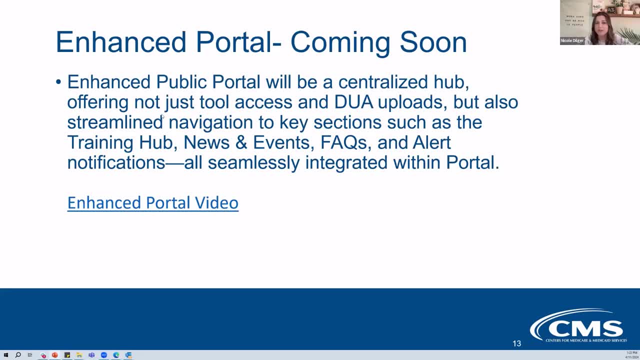 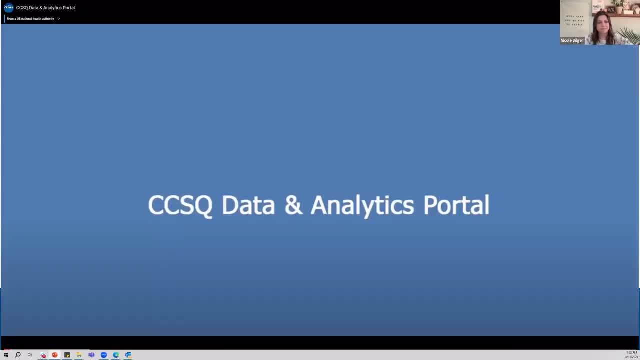 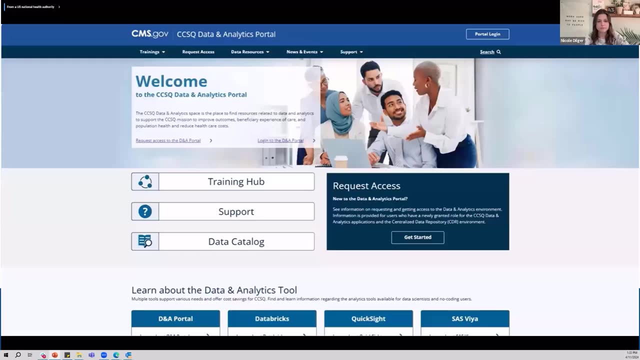 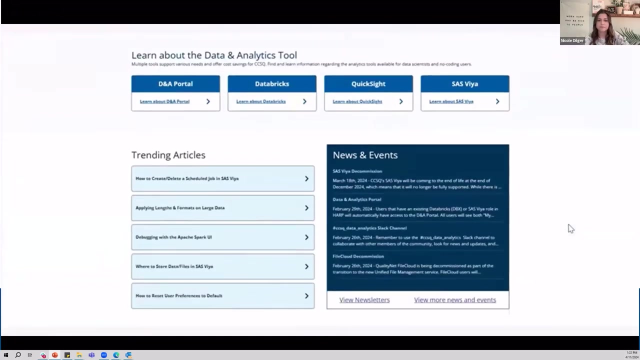 So very excited. Let's go ahead and play the video so we can give a little bit of a taste to everyone. The data and analytics portal transforms the way you experience and interact with our content. portal offers an enriched public content experience serving as your home for everything. data analytics. 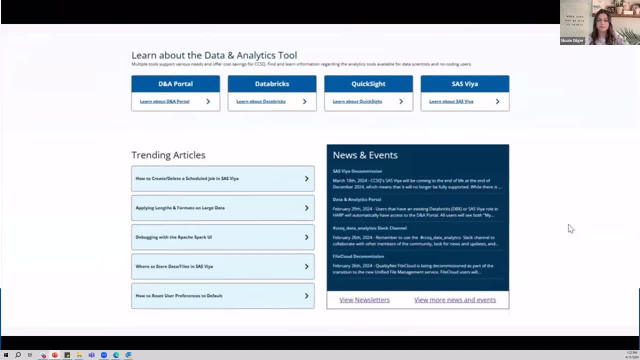 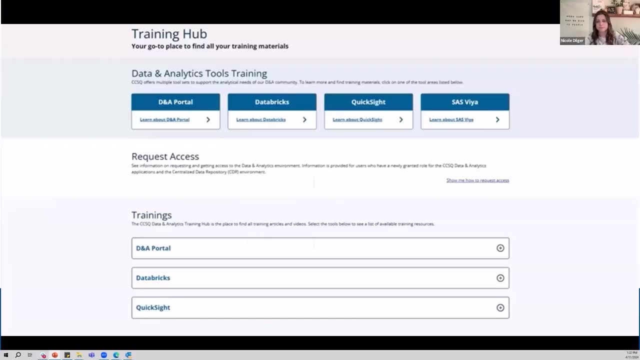 We've made accessing information easier than ever before And we've added features to meet your needs. The training hub houses your training resources, including knowledge-based articles and videos. Here you can find training materials for each tool set provided by CCSQ data and analytics. 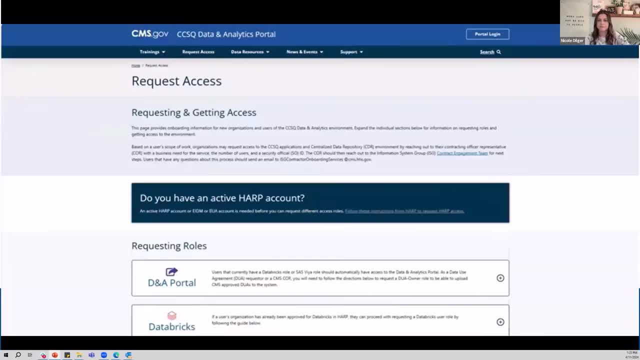 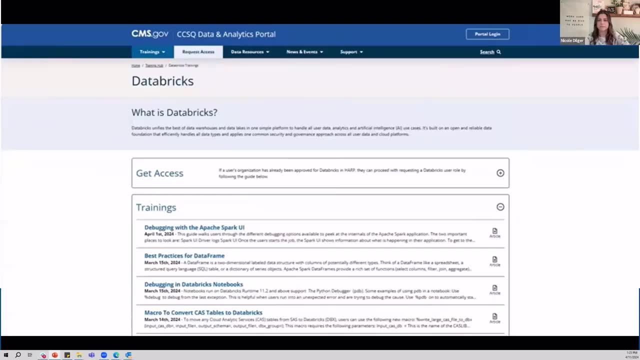 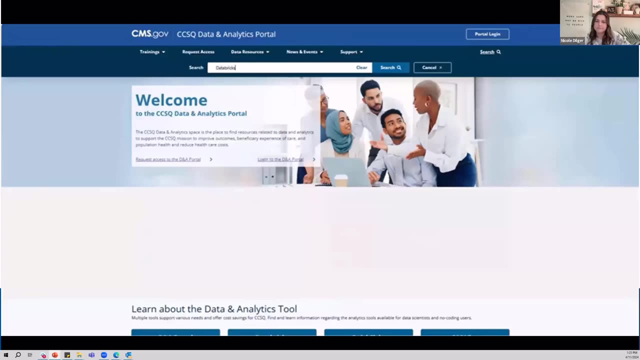 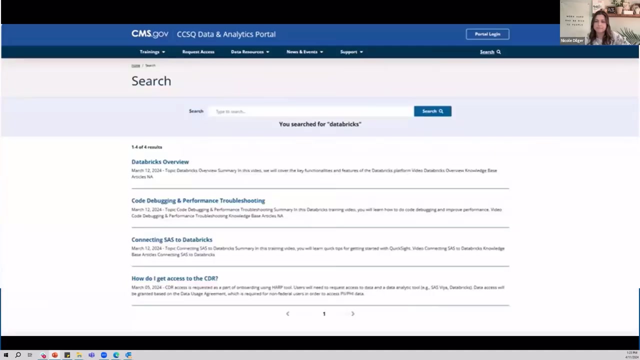 Additionally, you can request access to these tools through the training hub. Each training tool page offers a range of training resources comprising of a blend of knowledge-based articles and training videos. Confluence offered limited search functions. With portal, we've revamped the search capabilities, ensuring you find the right content quickly with its intuitive design and enhanced search capabilities. 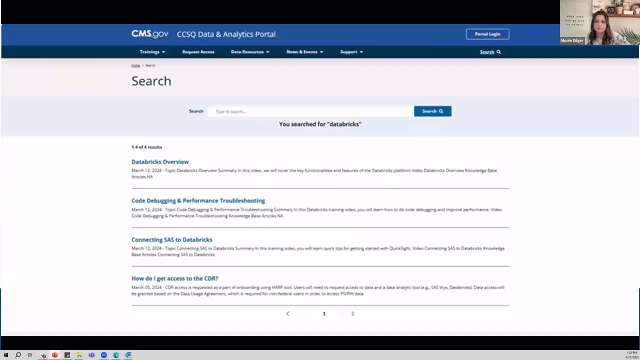 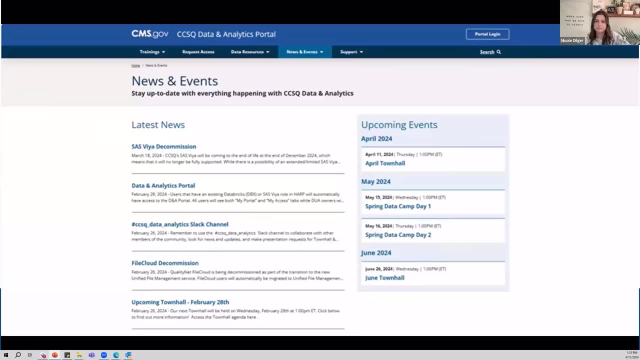 Finding the information you need is as simple as a few clicks. No more endless searching or frustration over buried content. Discover the latest updates and stay informed with our new news and events section. You can find information on happenings, including town halls and data camp. 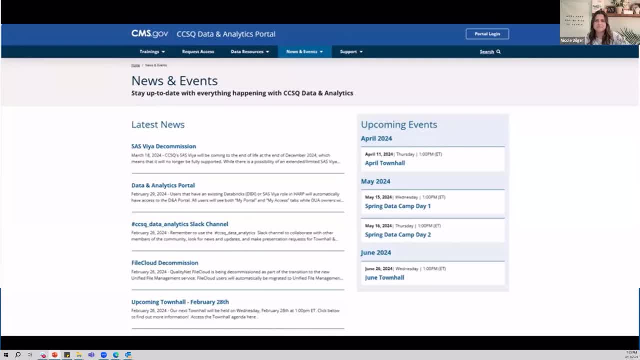 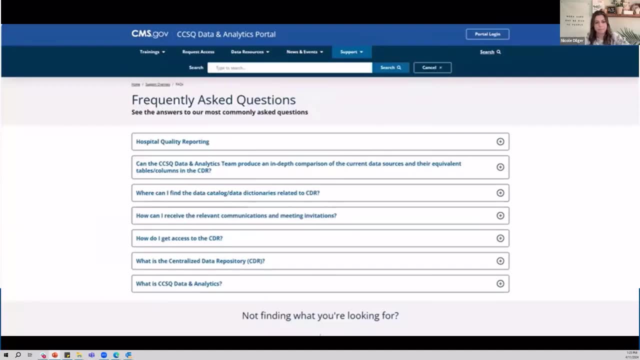 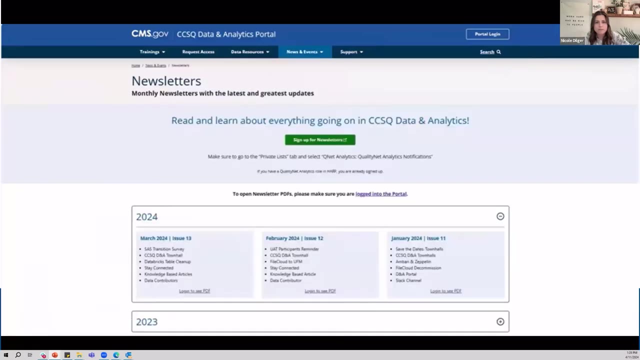 Check out news and events to stay in the loop and up to date with all that's happening in our community. The FAQ section organizes the most frequently asked questions. Whether you're curious about a topic or in need of troubleshooting guidance, our FAQ section will meet your needs. 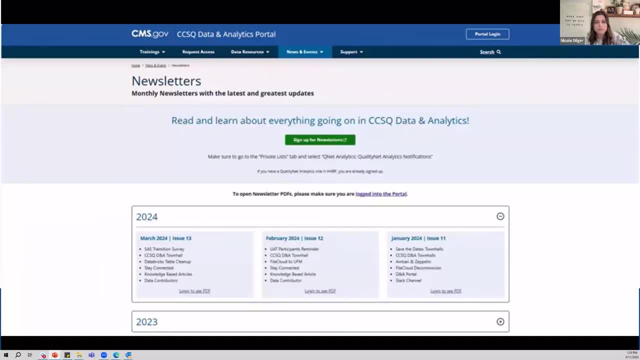 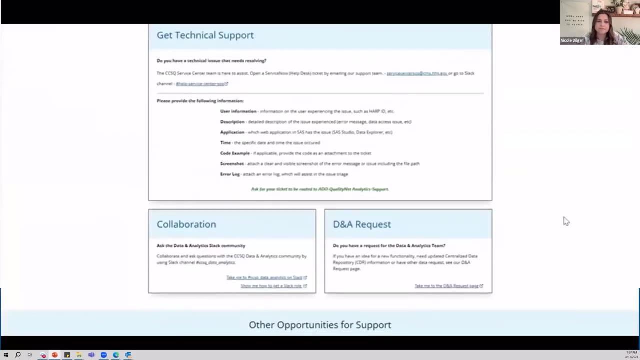 The newsletter section of portal brings all our current and past newsletters together in one convenient place: Newsletters, feature updates, training and important information. Browse the newsletter archive to catch up on anything you may have missed. Here you see another new portal feature. Our support section is your go to destination for all things technical assistance and data related. 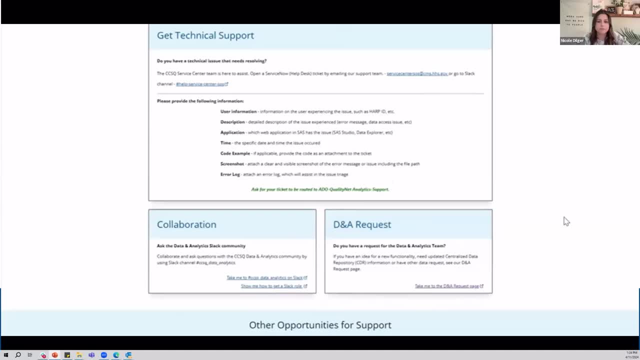 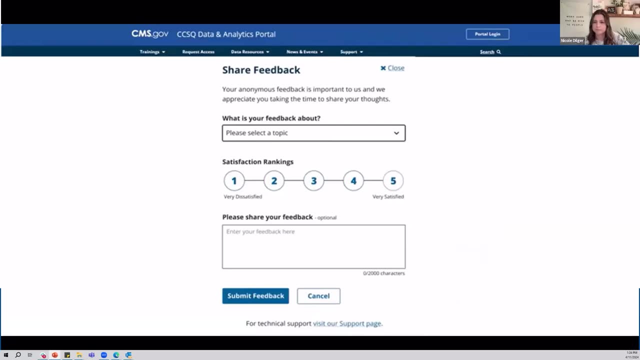 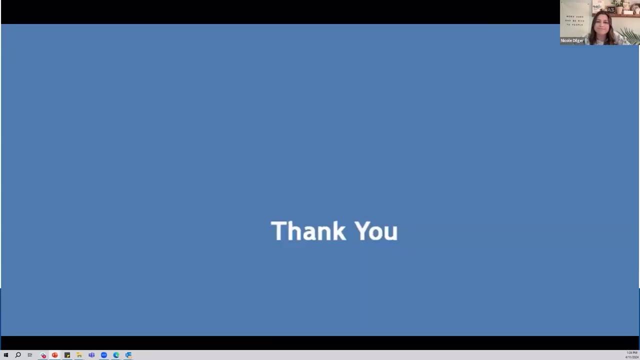 Whether you have a technical support request or a specific data analytic request, the support page can help. We value your input and in a future release you will have the opportunity to share your ideas and opinions using portal's user friendly feedback form. Thank you for joining us on this exploration into the CCSQ data and analytics portal. 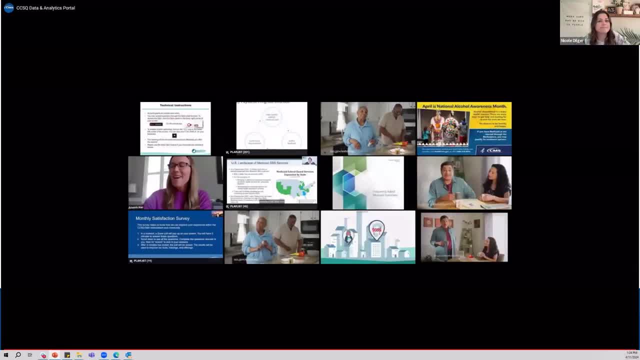 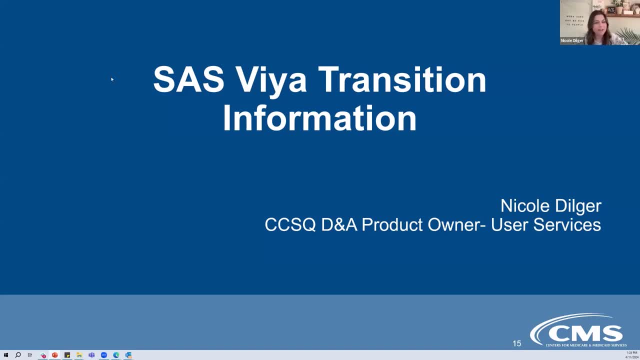 Keep an eye out for updates on the upcoming release date. All right, great. So, as you can see, there's going to be a lot of great things happening with the enhanced portal And, like I said, the release of that will be happening tomorrow afternoon into evening. 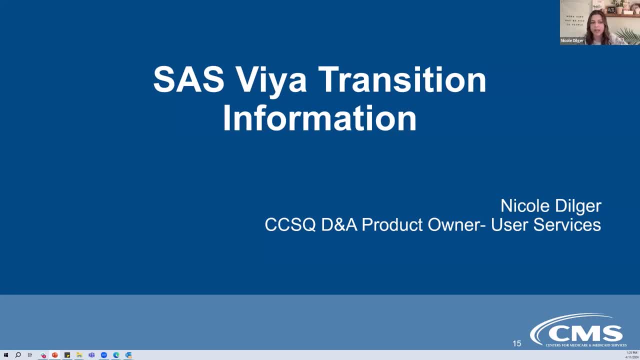 And we will be sending a communication out Monday morning just letting everyone know that that is up and ready to go. So let's go into our next presentation. So we're going to be talking about SAS Viya transition information. You can go ahead and go to the next slide. 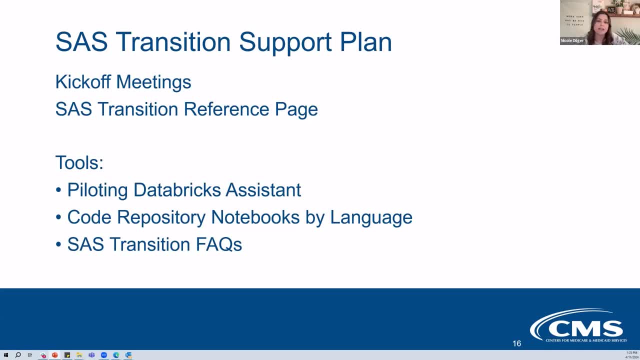 So what we're going to be doing is talking about the support plan. What all does that include? What does that look like to help the impacted orgs and users who are going to be transitioning from SAS Viya? So what we're going to be doing is, in the next week, you're going to be receiving an email related to scheduling kickoff meetings. 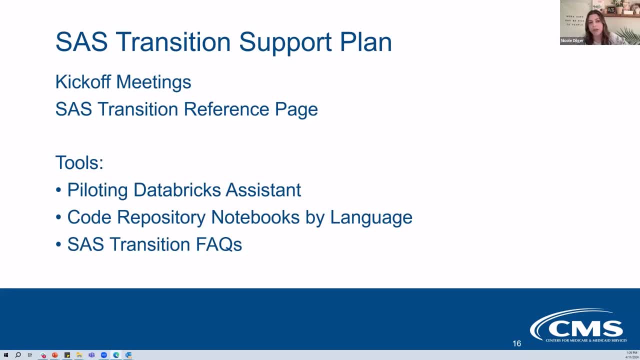 So there will be kickoff meetings scheduled with any impacted orgs who are currently using SAS Viya And those kickoff meetings will be starting as early as next week through the next six to eight weeks. after that We will have a SAS transition reference page. 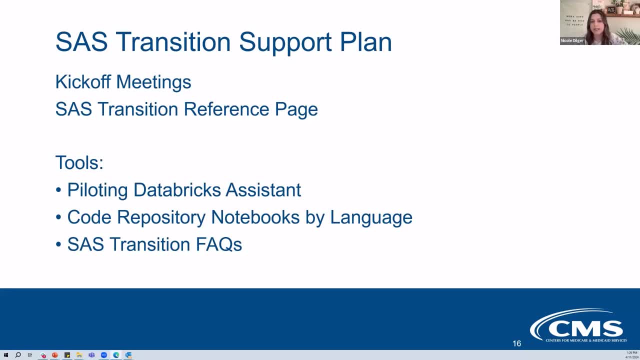 So kind of a one stop shop to talk about SAS transition, provide you with resources, training, links and instructions on how to access some of the tools which we have listed here. We're going to be piloting Databricks Assistant. This is a code conversion help tool that 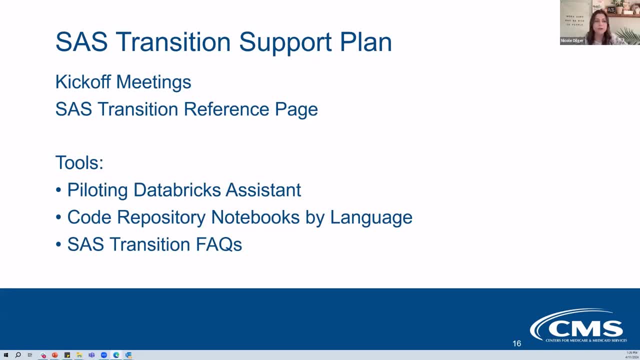 that is part of Databricks and we will be launching that in the coming weeks. You'll be receiving communications once that pilot starts, But that is exciting and will be available. We will also be creating code repository notebooks by language. Those of you that took the survey know that we had asked what language you anticipate you'll be using. 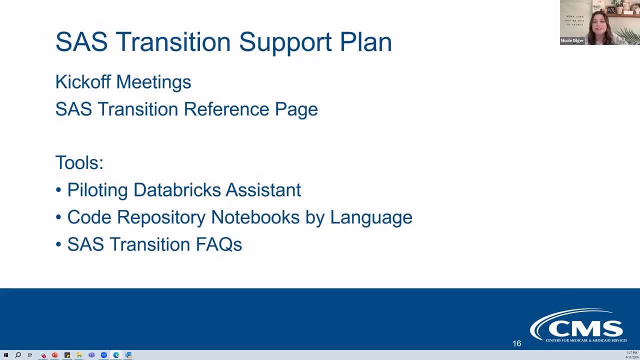 after the transition or during the transition. So we are going to be creating code repository notebooks by language to be able to help you in providing code snippets and examples, which we heard was something based on the survey that was going to be useful and, obviously, from feedback from users. 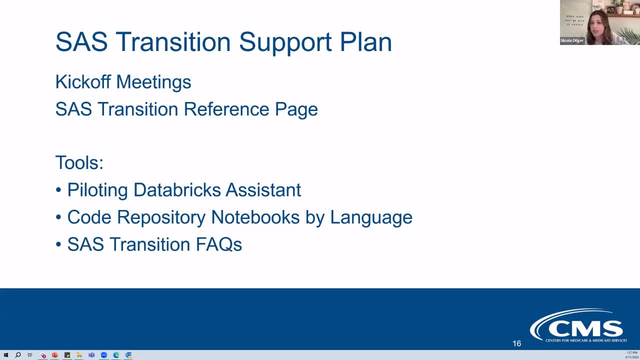 Additionally, we are going to have SAS transition FAQs. We've been compiling questions that have been coming in from different organizations and these are common questions that we feel other orgs may have the same questions. So we're going to compile them into FAQs and those will be uploaded in portal and 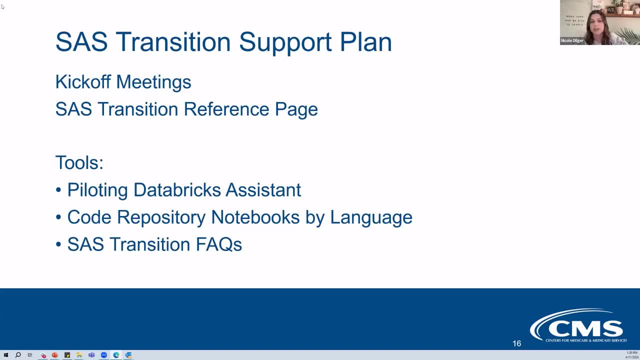 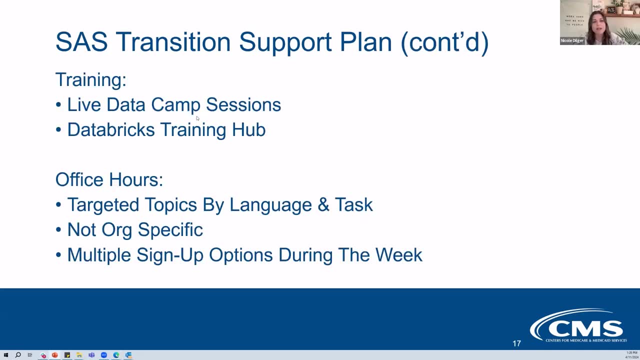 also linked on that SAS transition reference page that I mentioned previously. You can go ahead and go to the next page. So to talk about training, I know someone in the chat had asked about Python training. We actually do already have some Python training available in training hub. 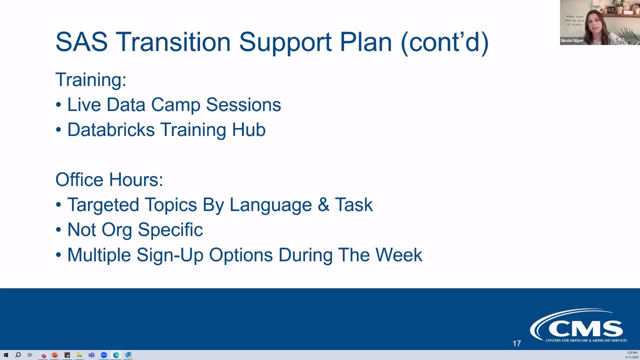 but there will be more coming. as you saw, with the upcoming data camp We will have day one of data camp almost fully covered or will be covering SAS transition. So a lot of those sessions are focused on helping the community transition off of SAS. 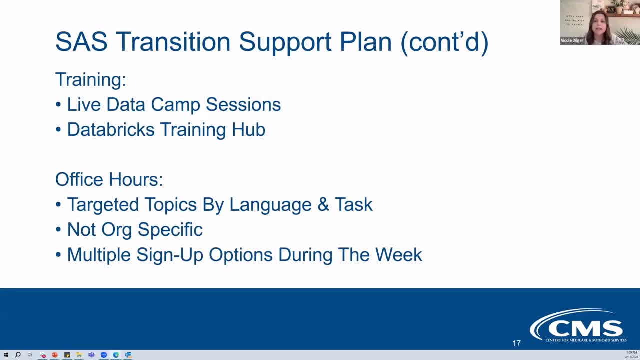 We will also have a Python live training there as well And, as Julia explained, we will be providing notebooks for those sessions in advance so that users can follow along, And we receive that feedback after the last data camp. So we're listening. We want to make sure that you have what you need. 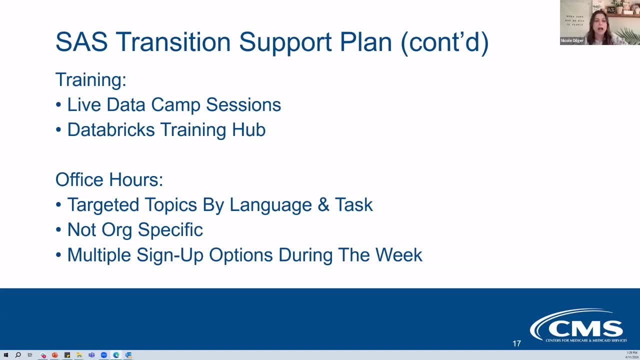 So those sessions will will be exciting. I mentioned the Databricks. training hub will continue to upload Knowledge based articles, training videos. make sure that those resources are available to you there and that you have what you need. And then, finally, as the last piece of our SAS transition support: 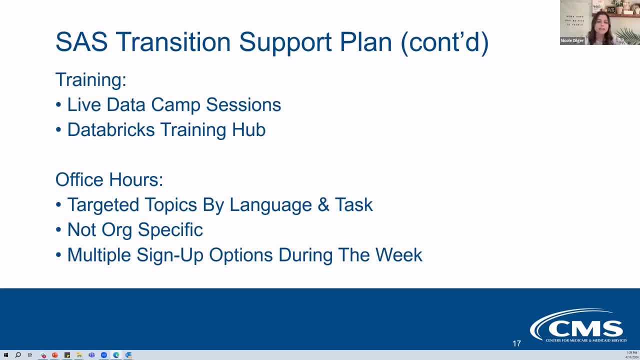 plan we will be holding office hours. This is going to be targeted topics by language and task, So these are not org specific. You'll be able to sign up. multiple individuals from multiple orgs can attend these sessions, based on your needs. So what we'll be doing is providing a schedule of what these office hour topics. 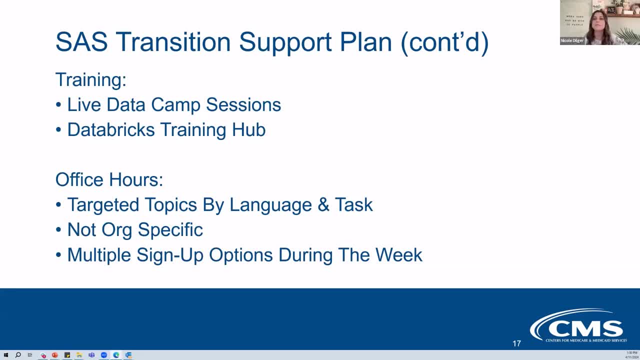 will be and when the slotted time frame is, And then you'll be able to sign up for those at your leisure. There'll be multiple sign up options during the week And we plan to cover the same topic twice, So if a specific date and time doesn't work for you, there'll be another option. 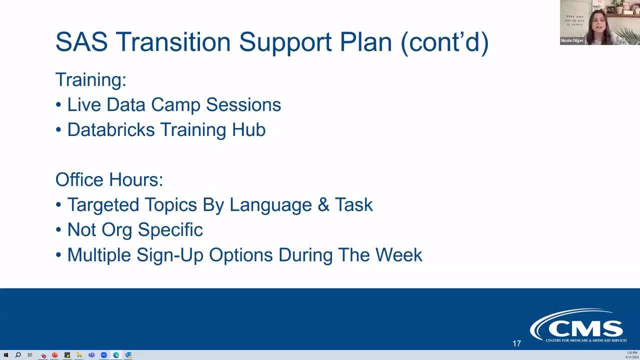 available to sign up for. So that is a recap of what our support plan looks like. As I said, there will be communications going out as early as the beginning of next week that will go into all of this information in more detail and also get those kickoff meetings scheduled. 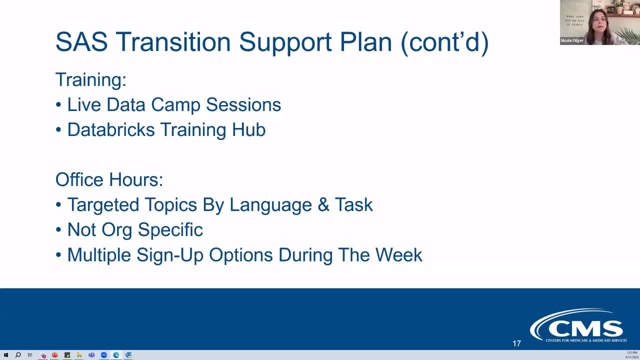 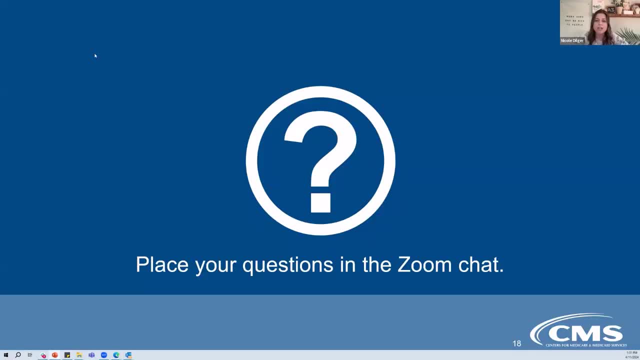 for everyone. All right, Julia, if you want to go ahead and go to the OK. so I think we're at. I think we're at Q&A now, So I'll pass it back over to Julia to go through what questions we have. 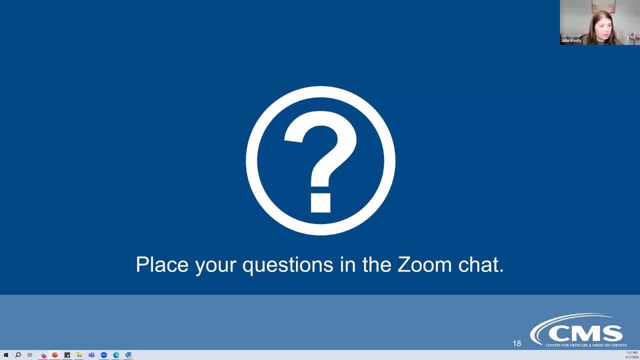 So I know a lot of our questions have been answered in the chat already. We still have a few. We have more coming in now. OK, so the first one that I don't believe has been answered yet, And if some of these have, I apologize for our team. 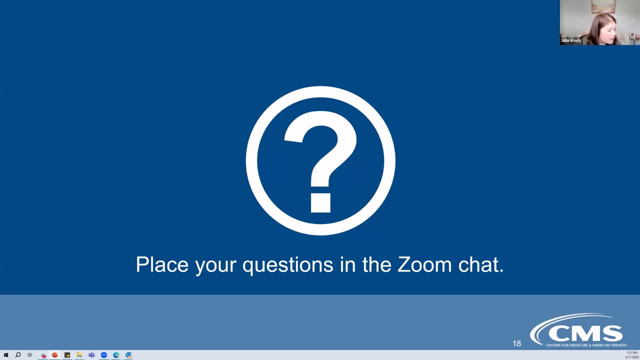 Please just let me know. Are there any updates for access to the HIVE tables using R? Julia, I don't have any updates on that. I don't know if anyone else from the team has any updates that they can share. If there isn't anyone on, we can certainly take that back. 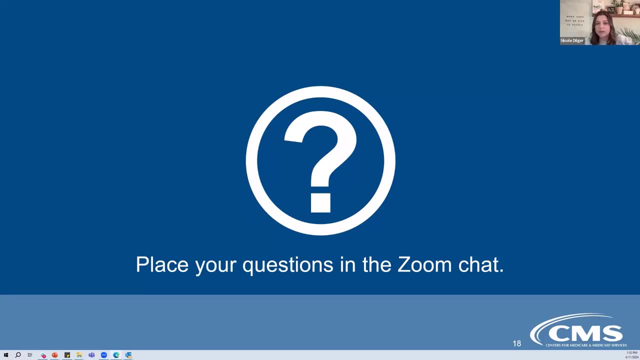 We take all of our QA and compile it and then make it available. So if we don't have someone on that can answer, we can definitely take it back and make sure that we get that question answered. Sorry, I couldn't unmute myself. 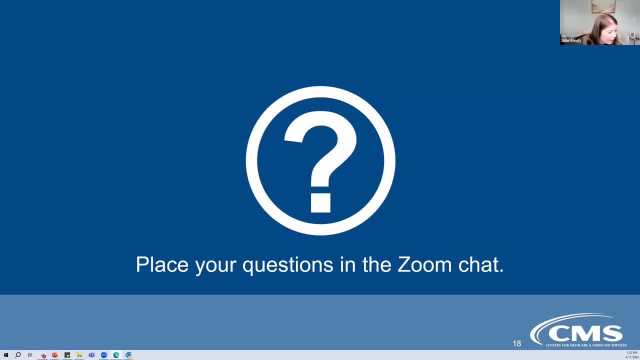 OK, that sounds good. Thanks, Nicole. OK, Justina, that's actually the one I was about to read too. SAS, MyUI- lets us see the um: all our internally created quarterly folders. Those are saved in our project dedicated to AWS S3 Bucket Workbench. 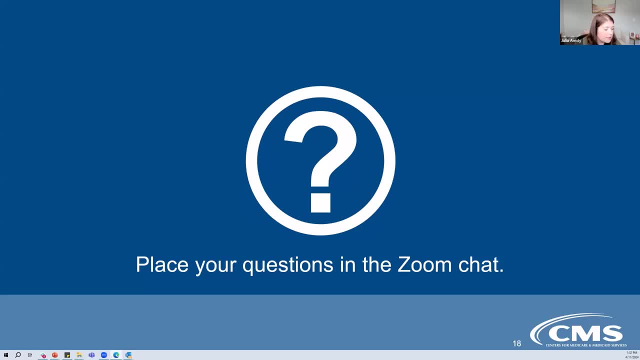 This helps us easily navigate through program logs, results and data sets Databricks, allows us to save data to the S3 Workbench, but doesn't have the UI to navigate folders slash data. Is there a resolution to this? SAS? I'm going to have the same response there. 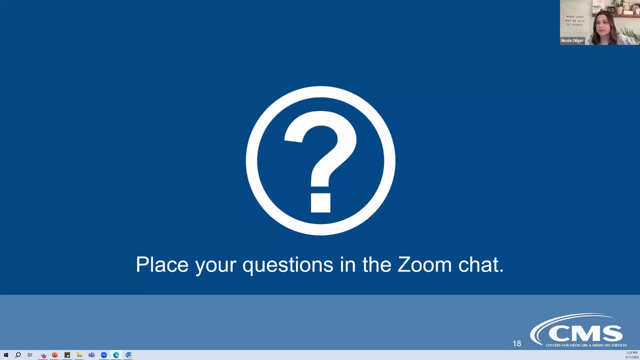 Apologies, I don't know if we, if we don't have our technical SMEs on, but I can't answer that question. but we'll certainly get get the answer for you all, SAS, And then, as Nicole said, after our town hall wraps, any questions that we just ran out of time for or didn't. 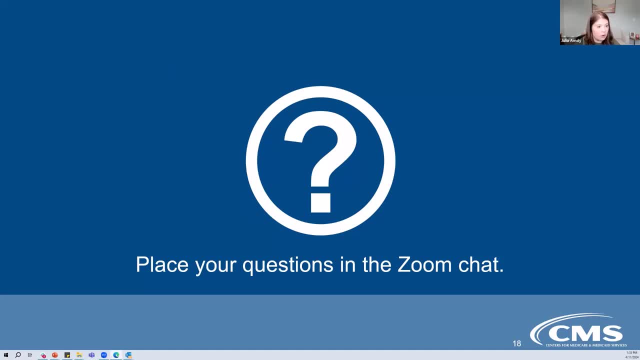 get to or that we're unable to answer. we don't have the specific people on the call for. We'll be sure to send that over to the DNA team. We'll make sure that those questions get answered And then all of the Q&A will be published with the rest of our slide deck and 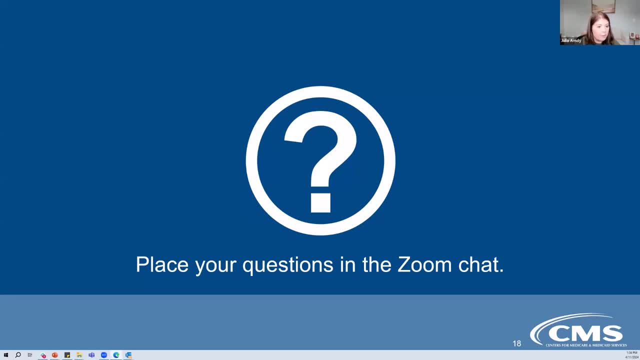 recording and that will be put on our confluence space. Aaron, I see you have your hand up. Yeah, I was struggling to come off mute to help answer that last question. So Databricks has a future feature called full volumes that will give us the ability to do that. 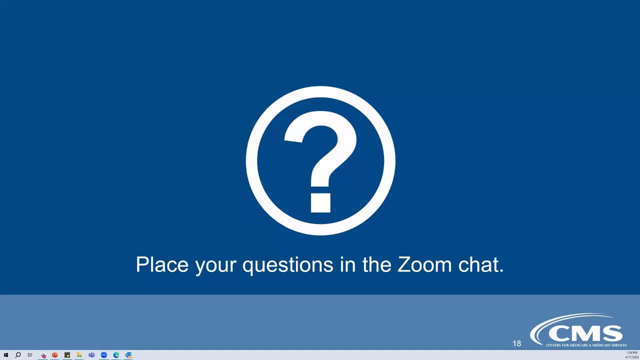 We have a couple stepping stones to get there to ensure that we maintain backwards compatibility and compatibility with SAS and that kind of stuff that prevent us from getting there right this minute. but we are working very proactively at enabling that. in the meantime, you know that work or that workspace is pointed to an S3. 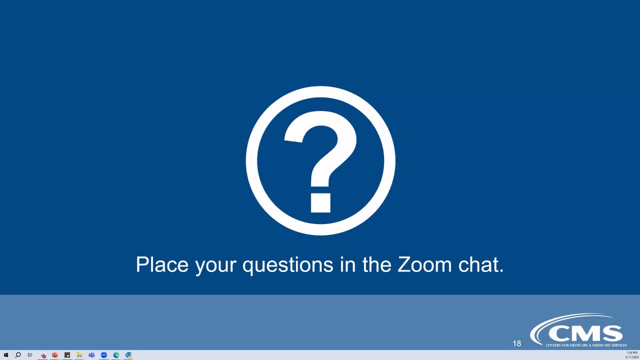 bucket. that should look very. it should be the same one that you can see in UFM or MFT or whatever you're using on that side. I can't remember what the I think everybody's moved to UFM at this point, but you should be able to do that there. 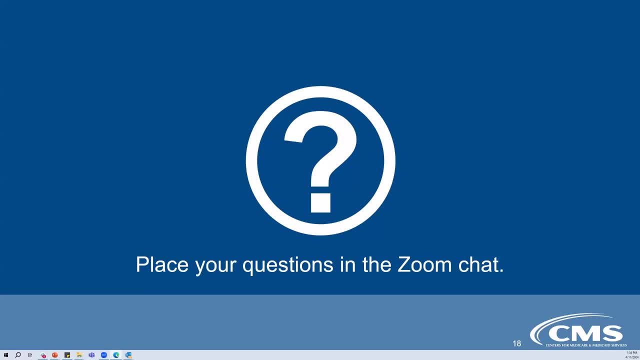 It's not the most ideal situation to have to kind of use two different tools to browse, but it's something that we are actively working on enabling in Databricks. Thanks, Aaron. Okay, so our next question, just to confirm the Databricks. 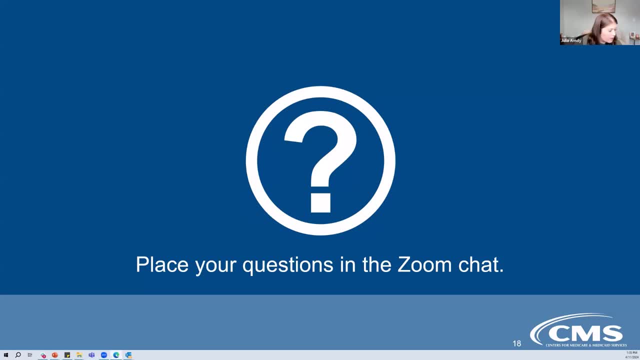 requirement is available now. right, So we can work with trainers to transition our SAS code to SQL. Sorry, I mean I was trying to get off mute and also responding to someone's question. So yes, Databricks is available, depending on if you are a member of the iQIES team. 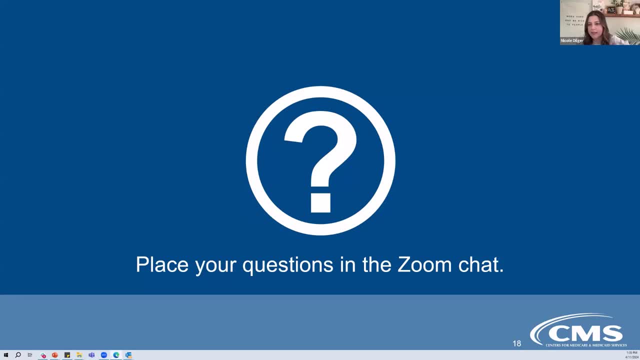 There has been a separate communication related to iQIES team members, who may not have access to Databricks, But if you are not part of the iQIES team, access to Databricks is available. Thanks, Nicole. And then one question we had was: 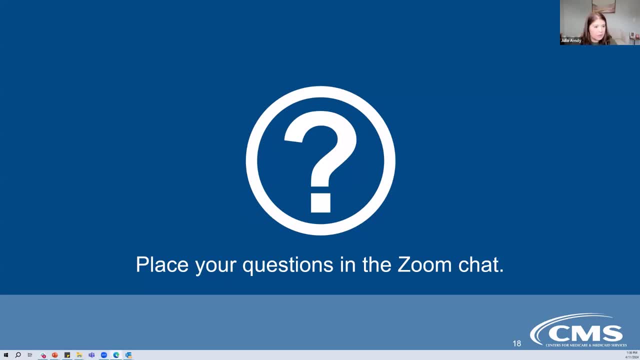 what is the link to the DNA portal? And correct me if I'm wrong. that's being shared out on Monday, So it remains the same. It's actually the same as it is now. We can get that put in the chat. It is the same link as we currently have for DUA owners to upload DUAs. 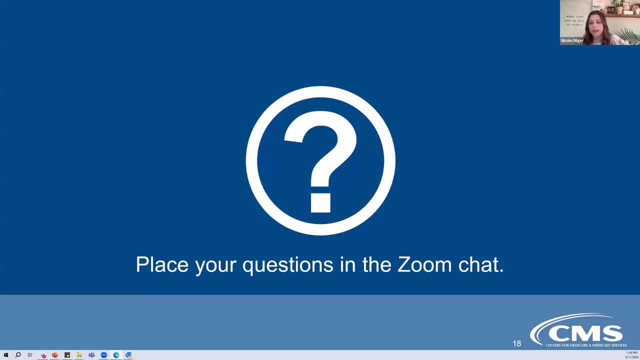 So it's not changing, but we will also include it in the communication that's going out Monday so that you all have it. And then is the support page of the DNA portal a replacement For ServiceNow. They can both still be used interchangeably. 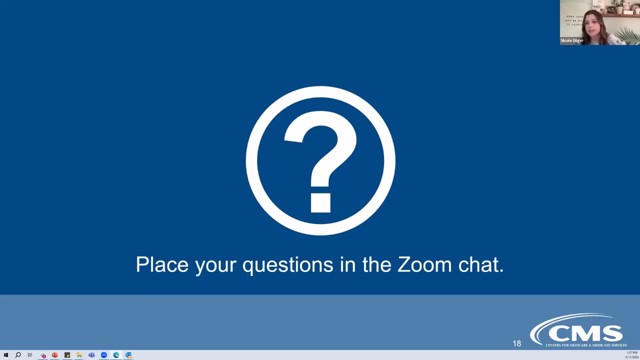 So if you have a ServiceNow, if you have ServiceNow access, you can still go in and submit a ticket, as you have done in the past. The support page: we have one on Confluence now where it just goes over different ways to be able to contact support. 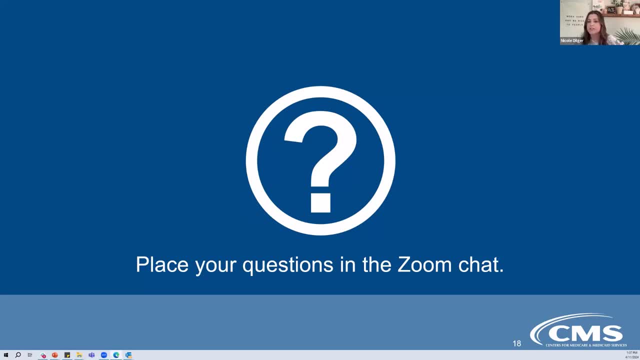 So, as an example- those of you that have Slack access- there's actually a, there's actually a help channel through ServiceNow that is available for Slack users. So there's a couple of different ways to be able to submit a help desk ticket that gets routed to us. 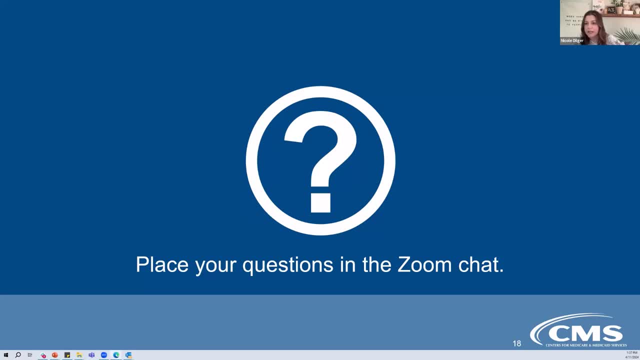 So that support page it can be utilized. in addition, if you already have ServiceNow access, Thanks. Is there a timeline for ability of utilization of job clusters and workflows? Can you repeat that question? Julia, Sure, no problem. Is there a timeline for ability of utilization of job clusters and workflows? 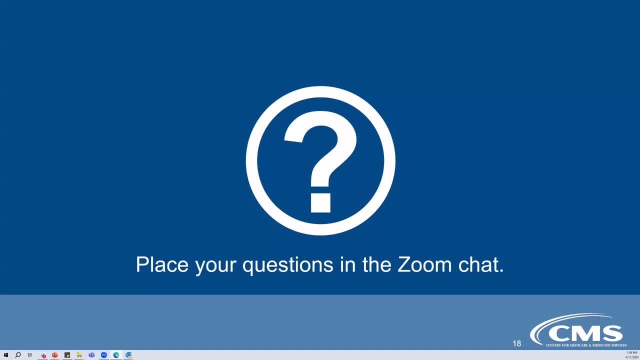 That one is definitely on a roadmap, just needs to be prioritized, which we don't have an active date quite yet. Okay, thank you, Sorry, I'm simultaneously trying to make sure I'm not missing any questions. Okay, are there resources for the difference? 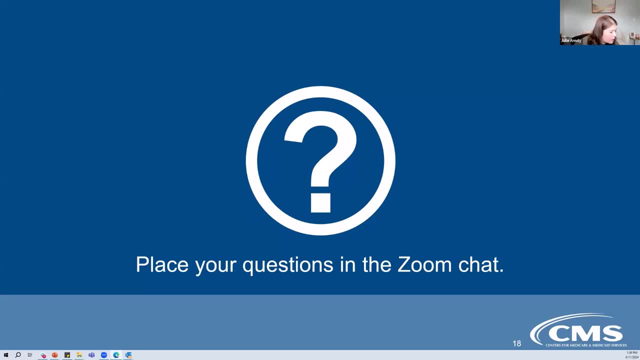 between base R and Python and the Apache Spark variations- Spark R, Spark L Y R, PySpark used in Dataverse. Yeah, was that was the first part of that. is there current training or documentation? was that the first part? 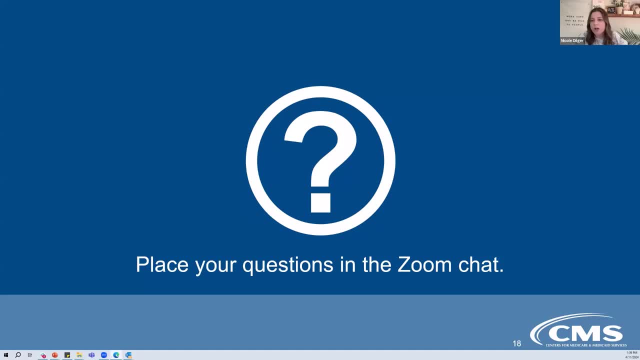 Are there resources? are there resources? Yeah, so part of that will be covered during data camp. We don't- I don't believe we currently have anything published. I'm trying to remember if, during this previous data camp, if that, if that was covered in one of the presentations. 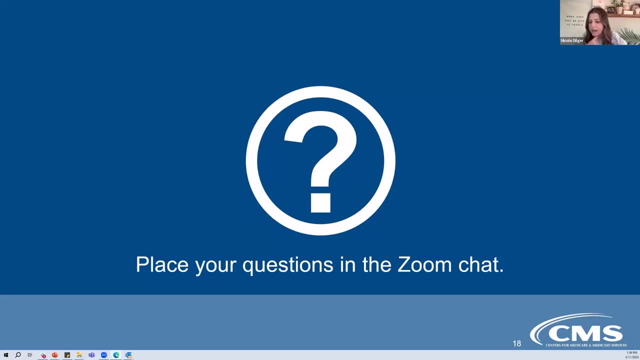 But we can definitely double check and then supply the link to that training video if so. But they do know that that is on the radar to be discussed during data camp. How do we connect MFT to Hive to load local tables? So you should have. every organization has their own workbench. 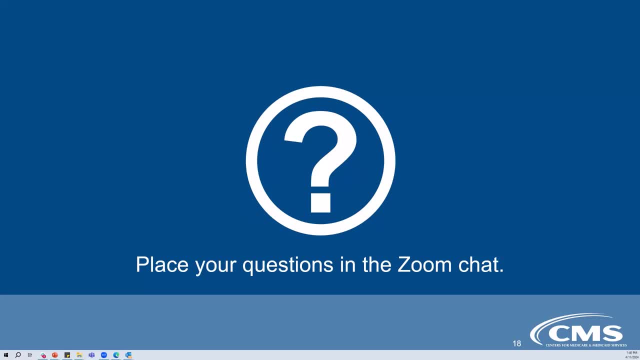 which is the same workbench that you access with SAS, which should be enabled in MFT. So you should be able to use FT to load and unload data into that workbench And then, from that S3 path, load or unload data into Databricks for use there. 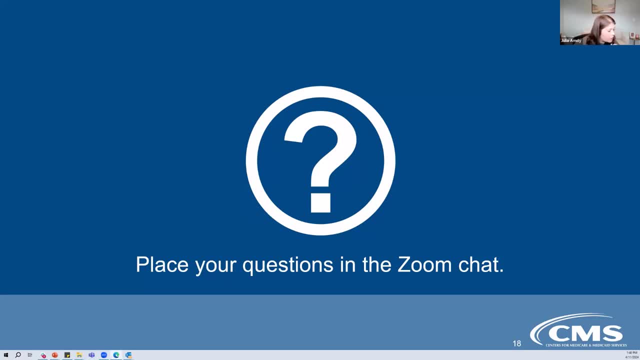 Okay, thank you, Aaron. Will MAX receive information on training sessions? My understanding is yes. I don't know if CMS wants to to chime in in anything additional there. This is Tom. MAX will definitely receive training and communication, Absolutely. 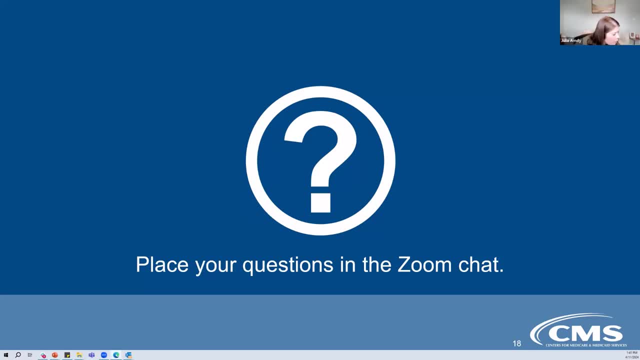 Thanks, Tom. Is the new portal a replacement of the current DNA Confluence or is it an augmentation of? That's a great question. So currently, when we release portal, Confluence will still be available. There won't be any changes to Confluence. 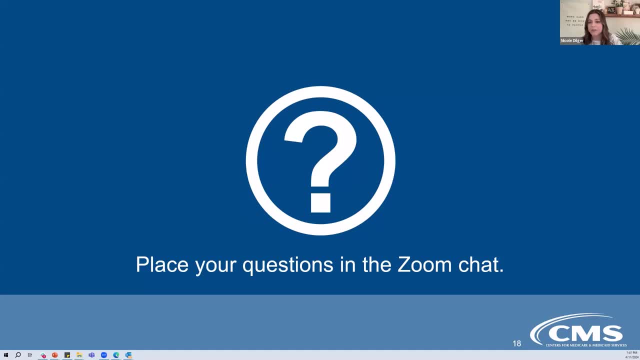 until probably one to two weeks after the release of portal. So majority of the content will now live in portal and will be archived in Confluence. There will be just a slight few items that currently live in Confluence that you will be redirected from portal to Confluence. 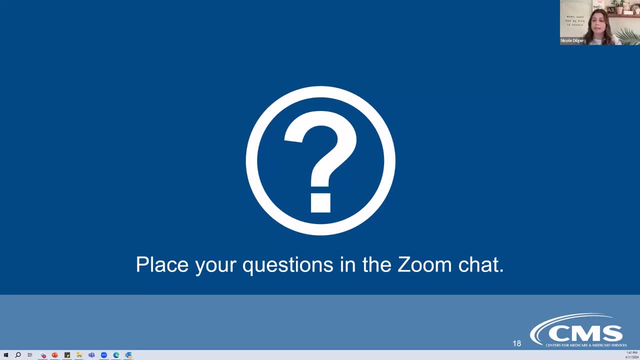 So if you're in portal and you click on data catalog as an example, that's going to redirect you to Confluence and pull that up as a separate tab on your screen to be able to review that. But for the most part it will be. 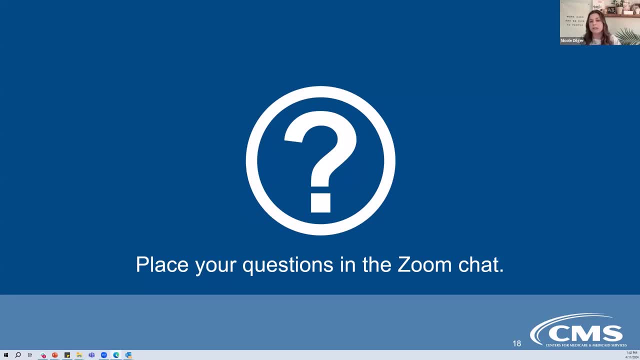 a transition of all of that information now living in portal instead of Confluence? Is it possible to create a shared folder in the Databricks workspace that multiple users can access and control the rights but would not be shared with all users? when I create a shared folder? 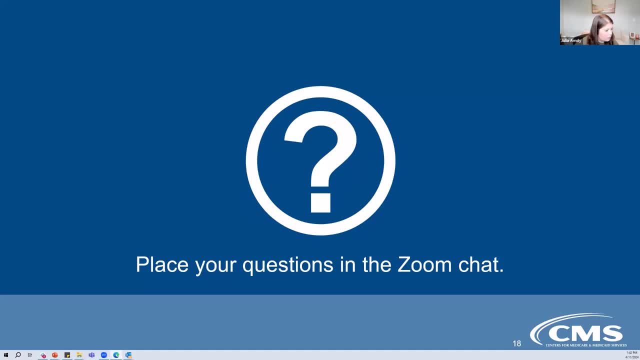 It must be shared with all users. Sure thing. Can you ask that one more time? Sure thing. Is it possible to create a shared folder in the Databricks workspace that multiple users can access and control the rights but would not be shared with all users? It sounds like currently. it says when I create: 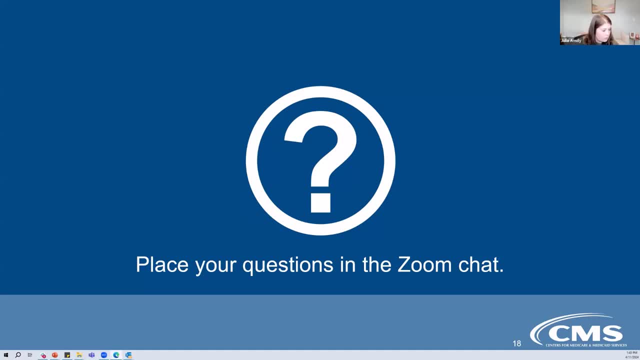 a shared folder. it must be shared with all users. But would it be possible to create a shared folder in the Databricks workspace that multiple users can access and control the rights but would not be shared with all users? Great question, We will have to take that one back and answer it all. 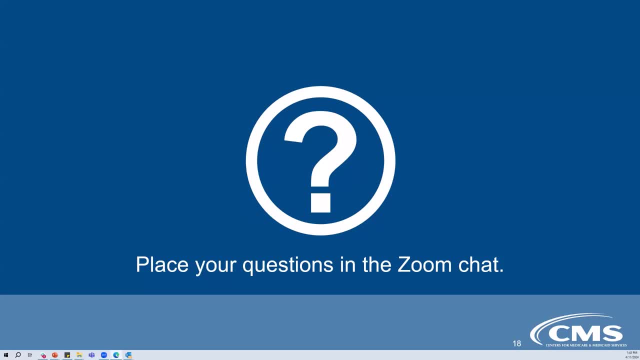 I see. Thanks, Aaron. OK, next is the Databricks coding assistant leveraging an LLM. If so, which LLM is the Databricks coding assistant using? Thank you, It is, It's a Databricks feature. 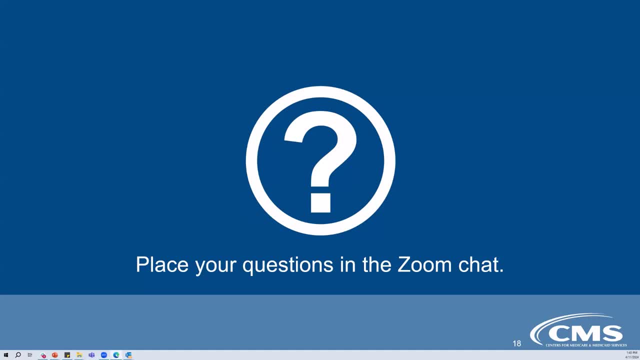 It's not necessarily given to us like what's running it, what's running it behind the scenes. so I'm not 100% sure. Databricks did just release a, you know, an open source LLM. I would presume that they're using their own, but I'm not completely sure. 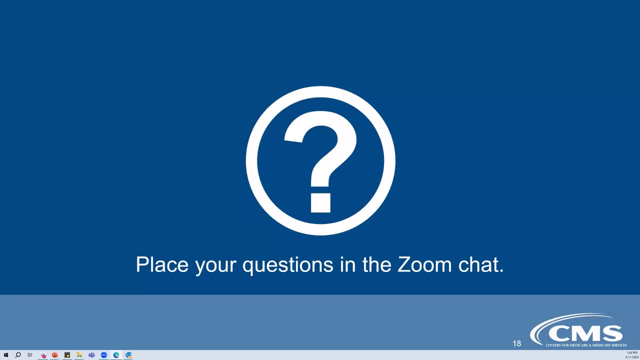 It's something we can ask the Databricks team. Thanks, Aaron. For individuals new to their roles, where is the best place to start to learn about data and access options? I would say that that would be our Confluence page, which will soon be turning into portal, but we can put that that link in the in. 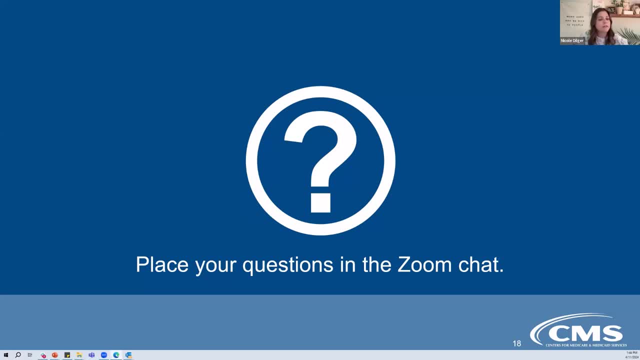 the chat. Will there be integration of RStudio functionality within the Databricks environment? I have to potentially get a little more information to know exactly what part of RStudio kind of is looking to be emulated, to be able to really answer that question. 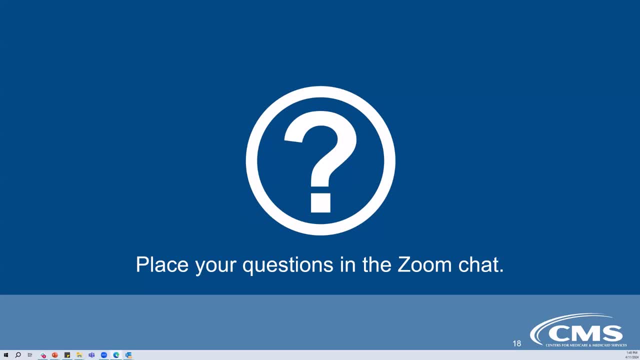 I think just ask kind of what exactly they're looking for. Hopefully they can follow up in the chat then as well. I'm getting an internet unstable notice. Nicole, can you still hear me? Yeah, you're still good. Fingers crossed, that stays. 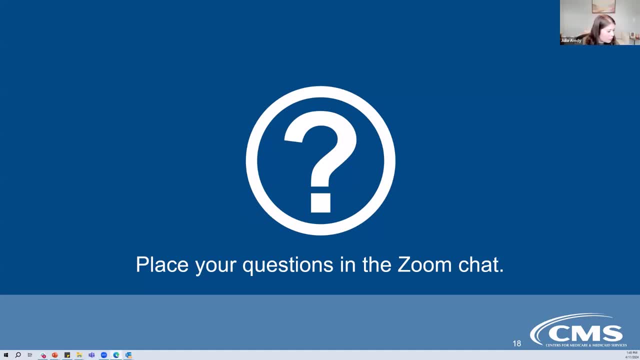 How do you use MFT to load? Are there instructions? And I don't know if who's on from the ESS team who manages MFT, But I'm. I think there's instructions on Confluence, but we can surely sync up with that team. 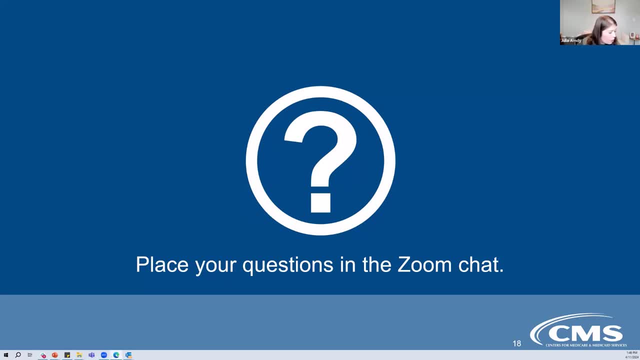 And then is there a possibility to be able to see all the files from the workbench on Databricks side on the Databricks side in the near future or ever? And then a follow up just says: I know, workbench file access is available. 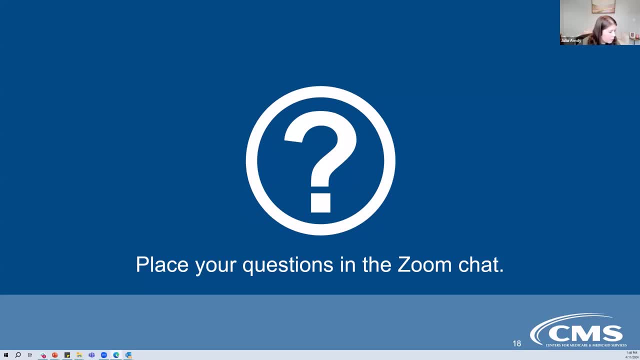 through MFT And we can also access and process them through our code on the Databricks side, but cannot see them on the side menu like in SAS Viya. Yeah, similar to the answer before on that one that requires Databricks volumes. 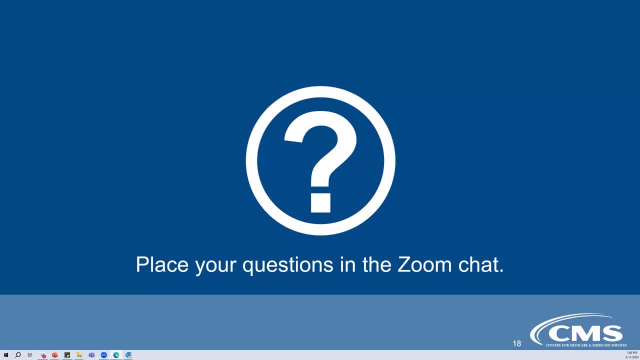 which we are looking at enabling, and there's a couple of different technical limitations that we have with our current architecture that we are looking at changing. It's one of those things that we are trying to step through- some backwards compatibility, and make the changes as little impact as possible on the end users. 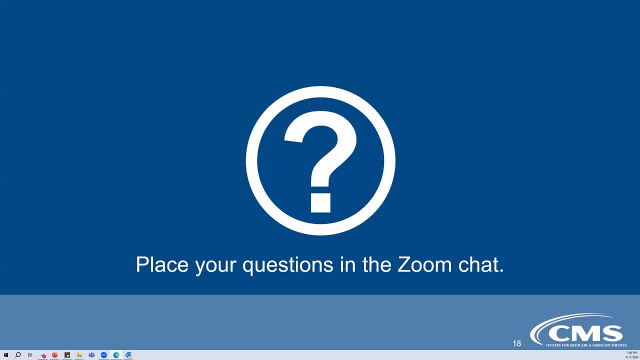 So we've got a little bit of. we've got a couple of things to enable that functionality that are slated on the roadmap And so I'm not exactly sure when that's going to fall, but it's definitely on a roadmap. Thanks, Aaron. 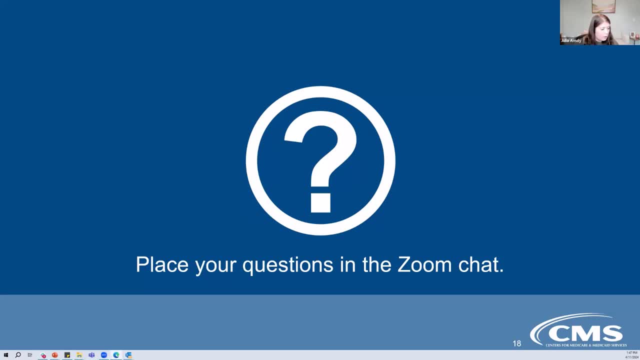 I'm looking back through our chat right now. I think at this point I've got all of the current questions. I just saw something come in: What are the current access control mechanisms for tables at the Hive table level for users? And then a second: is there any documentation available to understand these mechanisms? 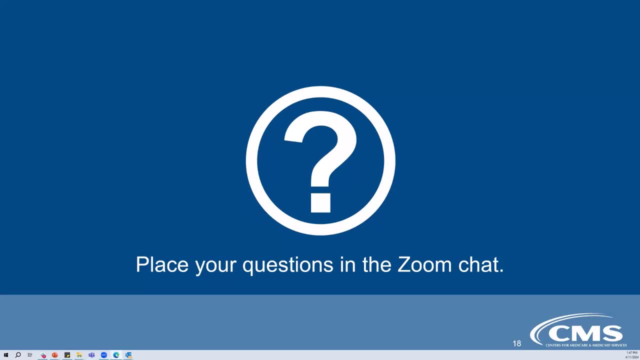 I missed the first part of that question. What are the current access control mechanisms for tables at the Hive table level for users? So everybody is apportioned a database for themselves which can be used in tables created. You'll have kind of carte blanche access to all of those that you create. 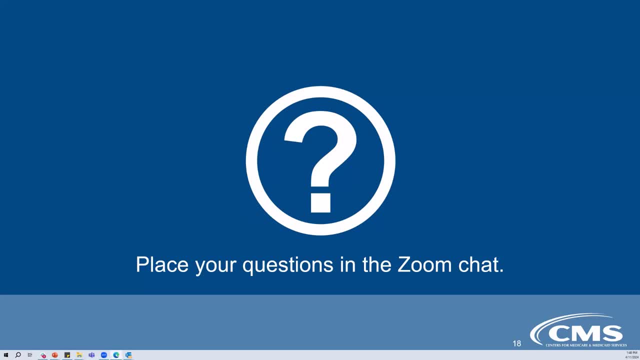 Other tables are managed either through the DUA process or, specifically. if it's not a data set that's actually governed by DUA, There's another process for that, And so we can granularly manage table access to any different org at this point. 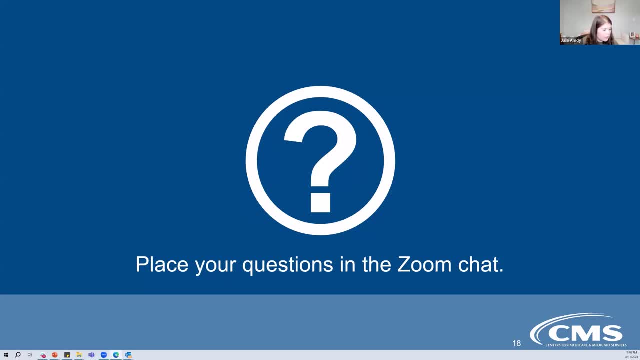 Thanks, Aaron. I think that I'm seeing some answers to questions coming, but I don't see any current questions. if I've missed any, please repost them in the chat Anytime. there's like a thread coming through. sometimes it gets a little wonky on mine. 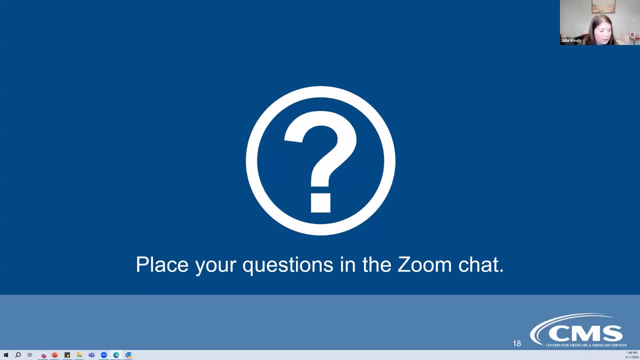 Is there a IMPL environment for Databricks and will the login process be the same? There is. However, we typically are not giving people access to that unless it's a BYOA access. So, like system to system, our IMPL environment is primarily for 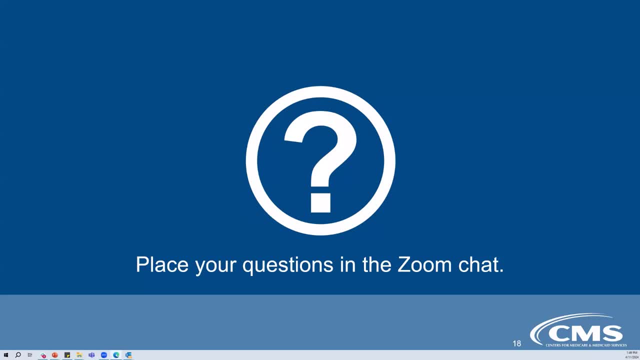 integrating other systems rather than user direct access. We're working on creating some of those databases that are not the actual prod database And so we're working on doing that by default, But really like, because Databricks is not like a monolithic kind of product that you can affect somebody. 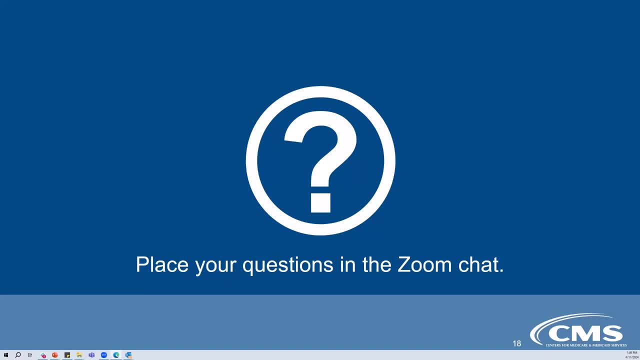 else. so typically for those kind of testing purposes we recommend that people use the prod Databricks. I mean kind of think about that as using the prod confluence right and managing and edit your data there, But like we're, and you can go to either a test table, not to interfere with any of 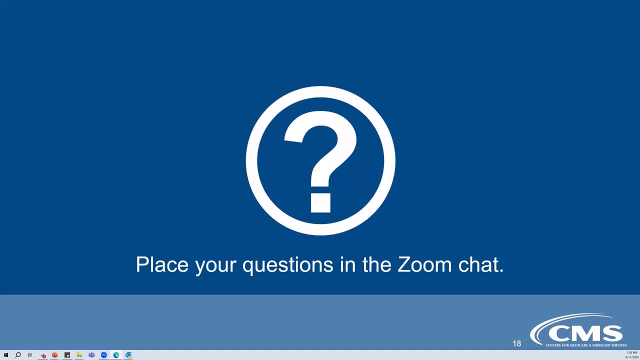 your prod tables or You can request a A test database be made and that will kind of be your container for any of your non production jobs that you don't want to interfere with. and typically people are trying to access prod data in our IMPL environment. 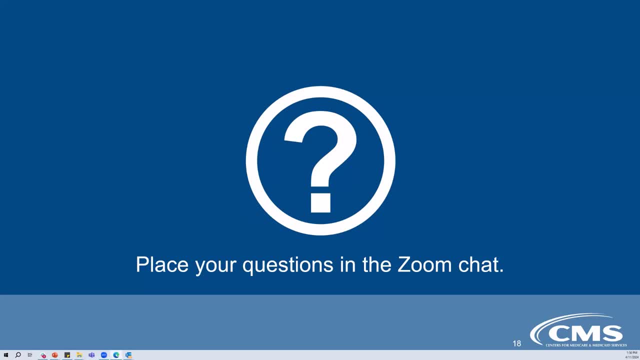 There is no actual data there. We have a couple like mock tables, but there's no actual data there. that will help you. OK, Aaron, it looks like that's an excellent response for you as well. Aaron said they have provided a structure for groups to put tables into. 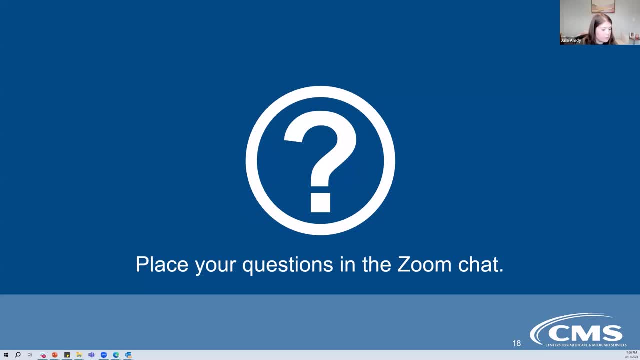 Is there a way to structure this, ie create subfolders within within it, to separate the tables into different folders? Yep, Yeah, So inside that workbench is up to you. The world is your oyster there, so you can create whatever folders you need. 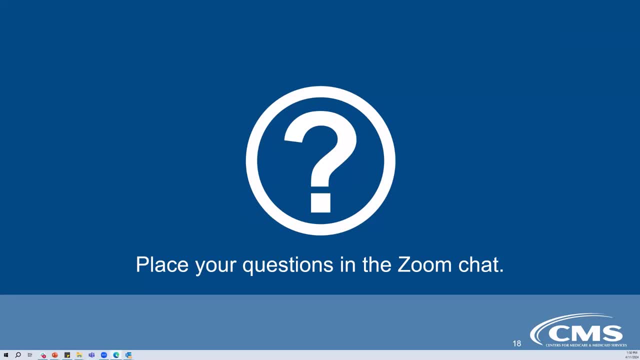 There is an effort- is- this is probably even too early to talk about, So forgive me- There is an effort to give a On production kind of lane in that, but we're still working on the exact specifics of it. but yeah, you can create whatever folders you want inside of there. 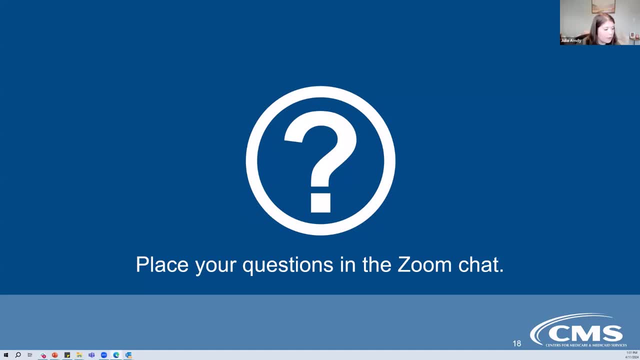 And, and then I did see I know we had a couple of people asking about how to use MFT to load our their instructions, and Gennady just dropped a link in the chat as well. so if anyone missed that, and then it looks like Jennifer Johnson also added. 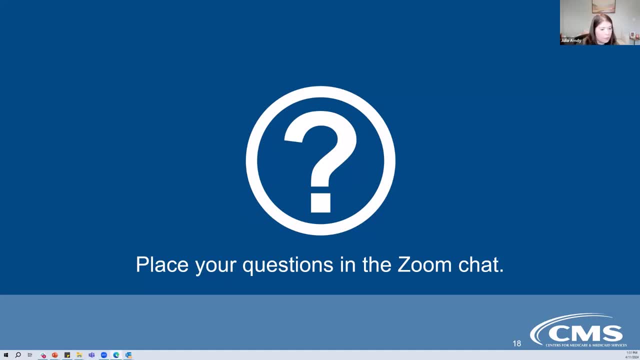 some links above to answer some questions, And then again, though, we'll make sure that all of that information shared is reflected in the Q&A section, But just in case anyone wants it immediately, it's there. OK, I think that is all of our just getting. one just came in. 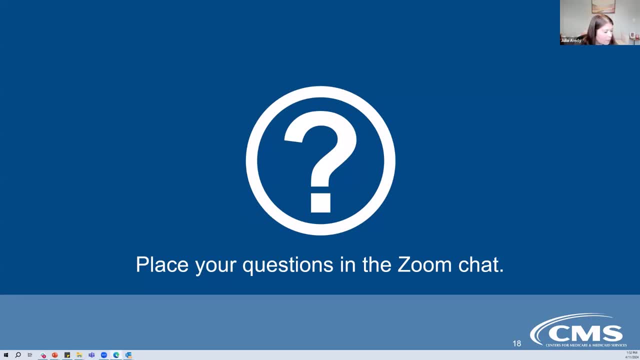 Were you asking about? it looks like in response to Josh's question, Megan was asking: were you asking about the high table schemas? And Josh said yes, So I don't know if that is a question still for Aaron, though I think Aaron already answered this. 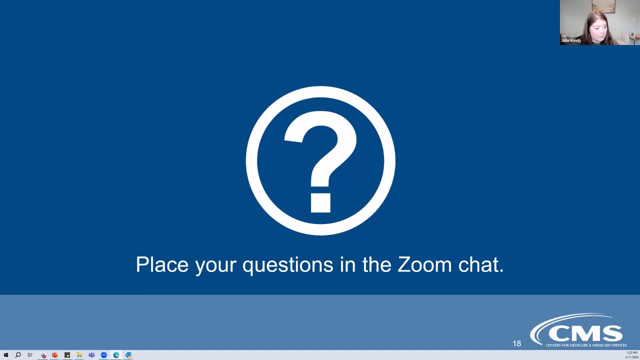 But I'm not sure. OK, I think at this point all of our current questions have been have gotten responses. Obviously, if anything is missed, please send it again, But if not, we'll make sure to get any that we didn't have answers for, or may. 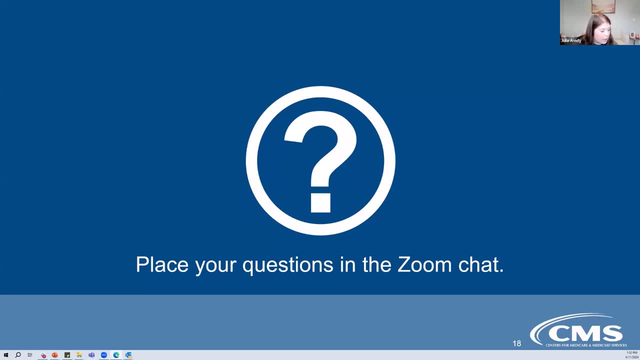 have missed out. as we got the Q&A answered, Here's another one. Are there any future plans to allow us, as users of the Databricks compute cluster, to install any library we need on the cluster, or all of the installations need to go through? a request to you guys. 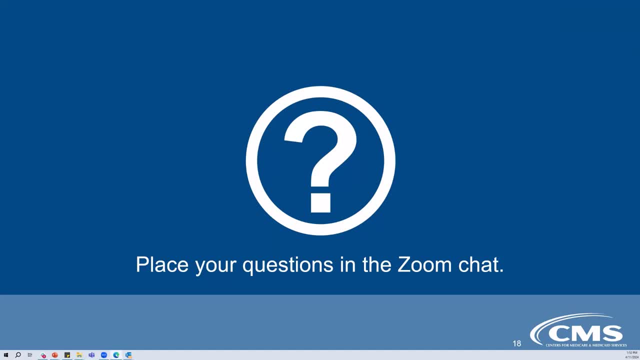 So you should be able to add whatever libraries that you want to your cluster After you start it up. acknowledging the fact that it is not the absolute most convenient thing to do that every time your cluster starts up, we are looking at some ways to facilitate adding those to kind of the default. 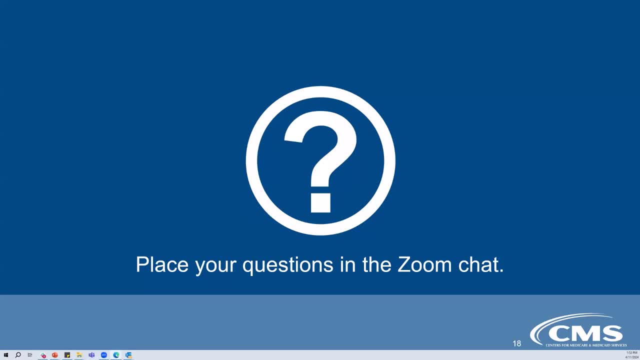 cluster, startup and generally. you know, we would also encourage people to use jobs as well, which you can kind of preload with those things, But right now you should have the ability to load the libraries that you need. Awesome Thanks, Aaron. 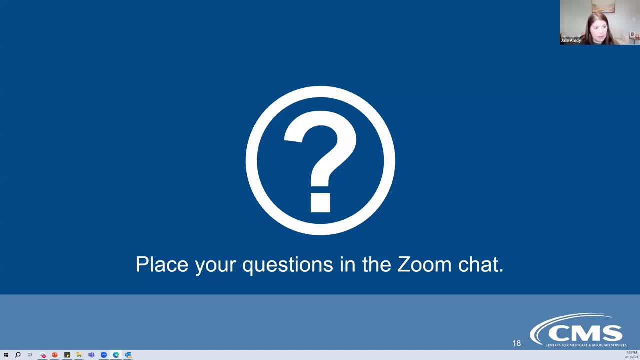 We'll give it another two minutes for any final questions and then, around 1: 55, we'll start turning it over. to wrap up, if a state agency is currently using SaaS to pull CMS data, will they be able to use Databricks for CMS data after the transition? 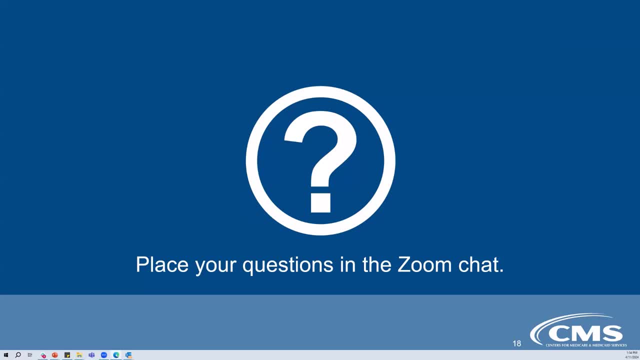 I'm going to yield to someone else who knows that I don't know. Hi, this is Justina. I'll attempt. I'm not sure if Tom Kress is still on the line or not, but at some point. yes, you should be able to, or you should be able to get the data via some other means. 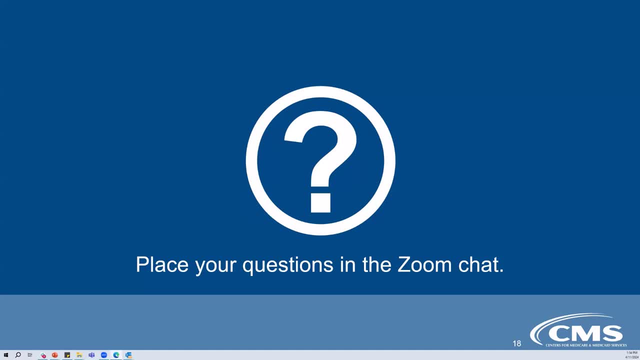 Right now. I know that there is a hall undertaken on the iKeys site that I unfortunately don't have details on. that may slightly postpone when you could use those tools If you would like to reach out to us and we can see whether or not we can give you the Databricks access ahead of time.